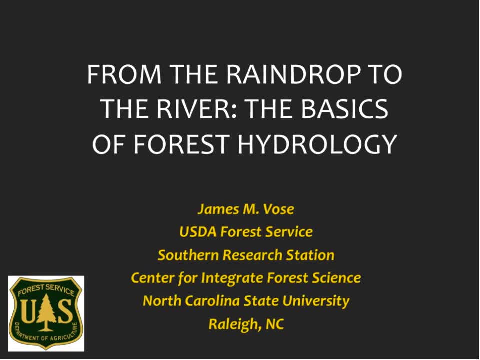 All right, Thank you very much. I assume everybody can hear me, okay. If not, let us know and we'll adjust accordingly. I appreciate the opportunity to speak with you by webinar today about a really important topic, and that is the relationships between forest and water. 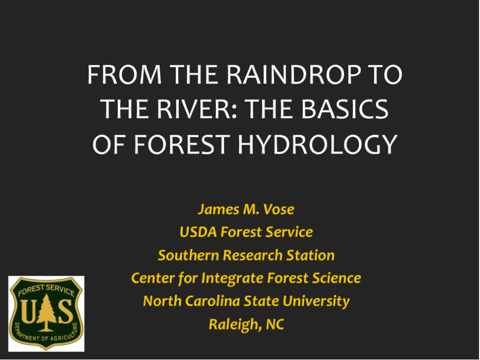 This is one of three kind of consecutive webinars that are meant to be connected. In about a month there'll be another one that talks about land use and landscape level processes and how those influence water resources, and then, about a month after that, one on best management practices. 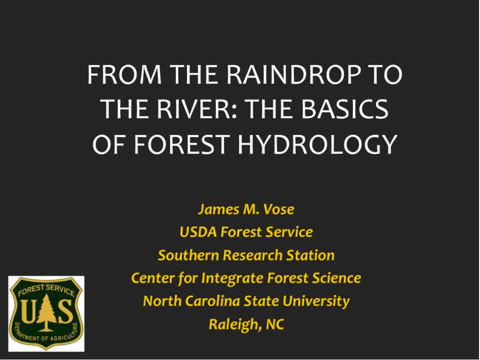 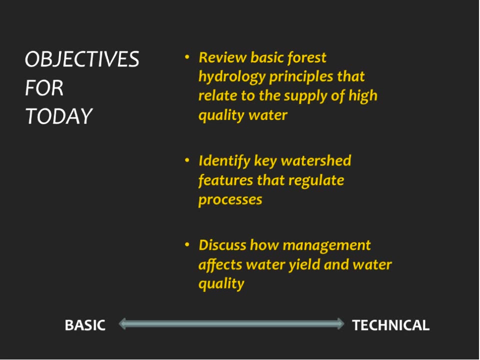 And this first webinar was an attempt to provide a bit of a precursor to those following ones, so I encourage you to stay tuned for the next couple that will be coming about a month out and then another month. So I'd like to do three things today. I'd like to first review some basic forest hydrology principles and focus on the ones that really relate to the supply of high-quality water. 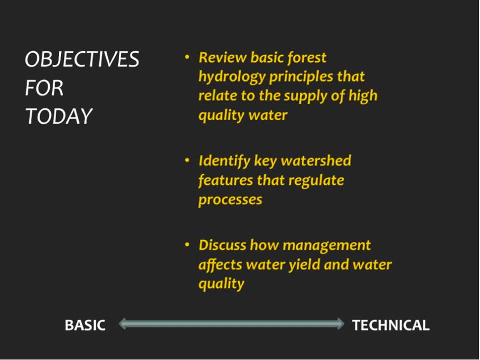 With that, I'd like to identify key watershed features that regulate important processes and then discuss how management affects water yield and water quality. And for the management, I'll primarily focus on forest cutting. And for the management, I'll primarily focus on forest cutting and prescribed fire. 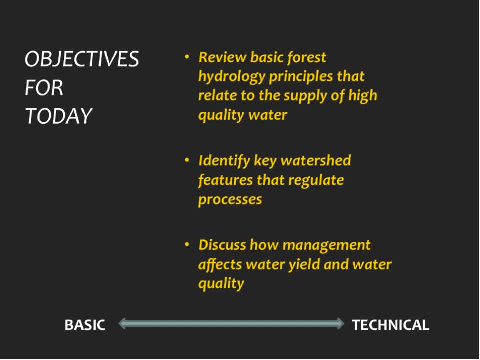 Now, this presentation is going to span the spectrum from very basic knowledge that you may have learned, or either in school, way back when, or through on-the-job training, But also I'm going to blend in some research and some highly technical information, So for some of you it may be a refresher of some things that you already know. 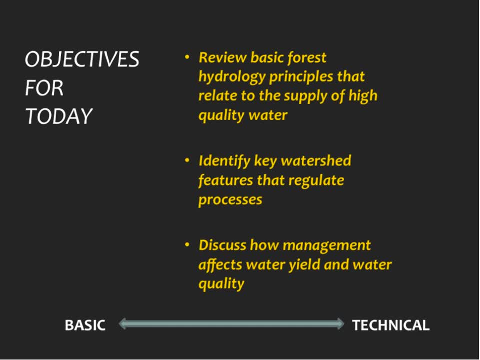 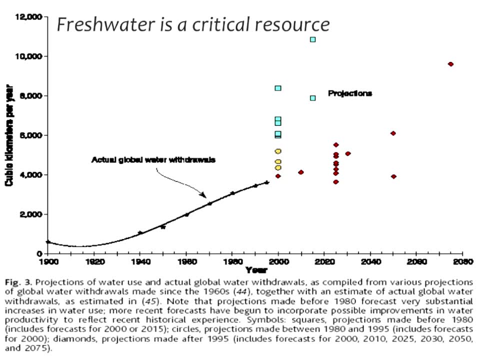 In others it will be new information that you perhaps have never heard before, But I think all in all, and I hope all in all, you'll learn something in the process. Now this is a slide that just shows sort of the historical trend in global water withdrawals and then future projections. 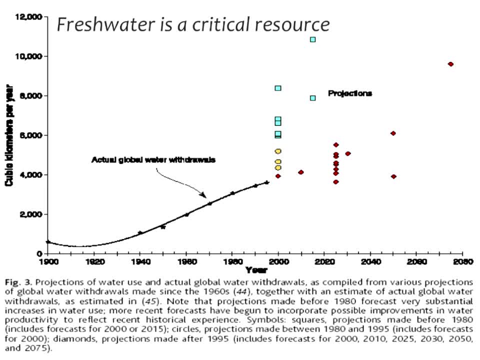 And the future projections have a wide scatter about it because it depends on population growth estimates and conservation practices. But the bottom line is: fresh water is a critical resource that's destined to become. but the bottom line is: freshwater is is a critical resource that's destined to become. 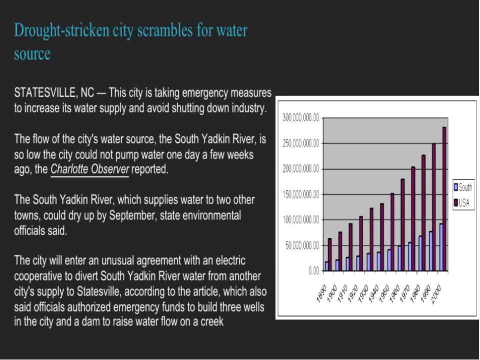 even more critical in the coming decades. Now it used to be that in many parts of this country in particular, there were areas that where fresh water was so abundant that most of the efforts were focused on trying to control flooding, and the notion that water resources would become scarce was further from most. 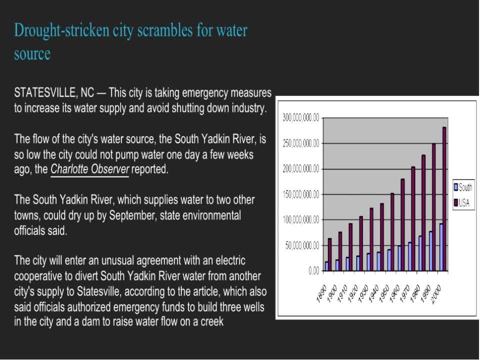 people's minds In many regions. now that's no longer true. This headline was from the Charlotte Observer in North Carolina, and this is a city, town of Statesville, that came within a few days of running out of water, And the reason that that happened is that the last few decades have been subject to 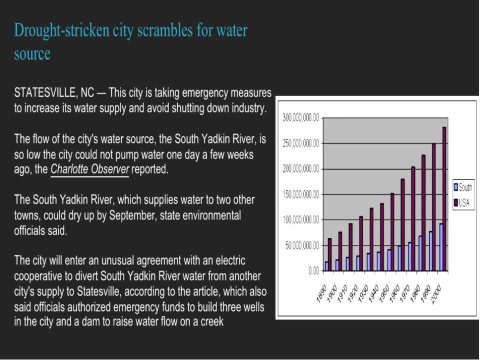 some serious droughts, but also, as the panel on the right shows, this is a region of very fast population growth, With the average person using about a hundred to two hundred gallons of water per day. Industrial and agricultural growth to support that growing population. this is a headline. 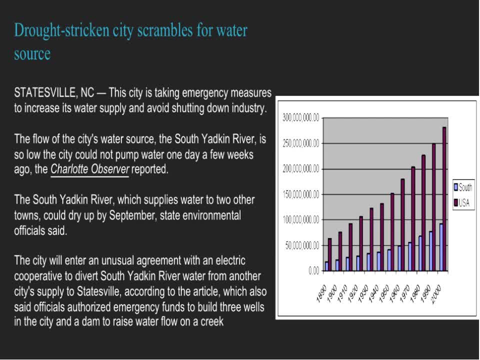 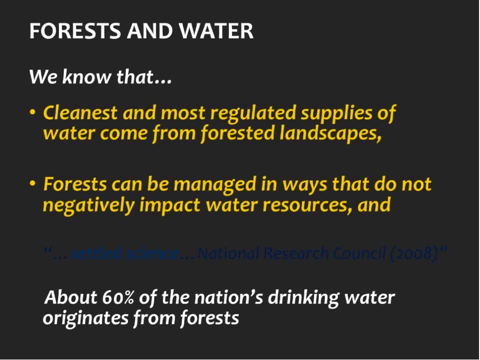 that's likely to be played out- and has played out since this headline time and time again. Now, the reason that we're talking about forests and water is that forests have a very important role to play in supplying water to aquatic ecosystems and people. We know the following two statements: 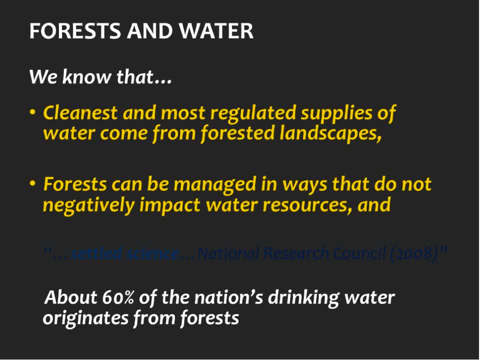 One is that the cleanest and most regulated supplies of water come from forested landscapes. We also know that forests can be managed in ways that do not negatively impact water resources, And this has been concluded to be settled science by a recent, fairly recent National 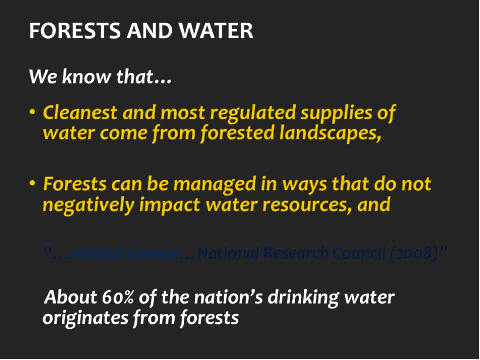 Research Council report And I will say that there's very few things in natural sciences or natural systems that we have this much confidence in, But this is one that is. It is And those two statements are recognized to be true, And it's a good thing that we know about that and a good thing that we know the value of. 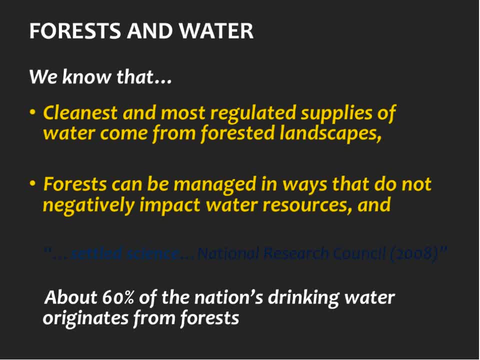 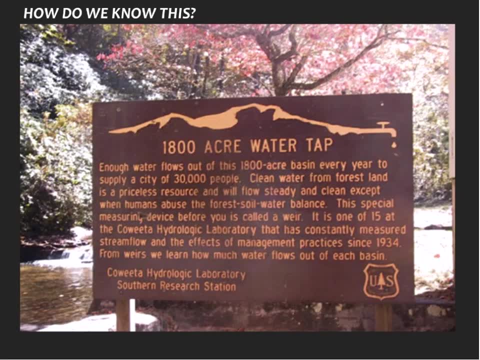 forests for supplying water, because about 50,- I'm sorry about 60%- of the nation's drinking water supply originates from forests. Now, how do we know this? Well, one of the reasons that we know this and one of the reasons that it is settled: 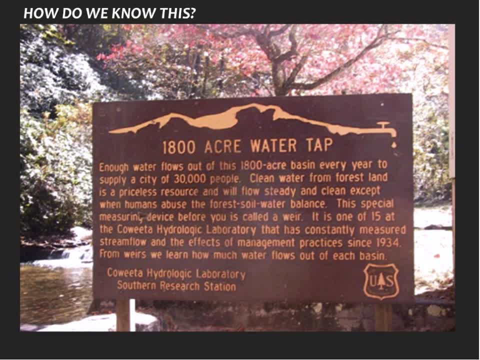 science is. this is an area that we literally have. decades of scientific information on The original origins of the US Forest Service in particular had a lot to do with the fact that land managers and the state of the science at the time recognized that there needed to. 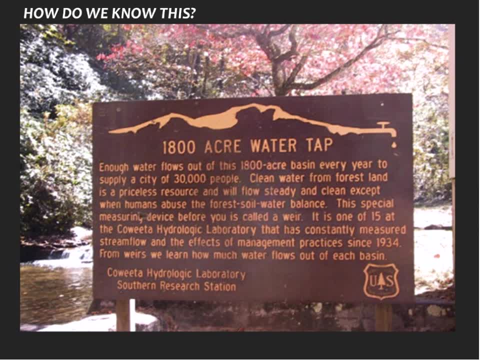 be more information about the relationship between forests and flooding in particular, But also forest management and water quantity and water quality. As a result, there were several experimental forest watersheds set up across the United States, And this is a good thing. This is a good thing. 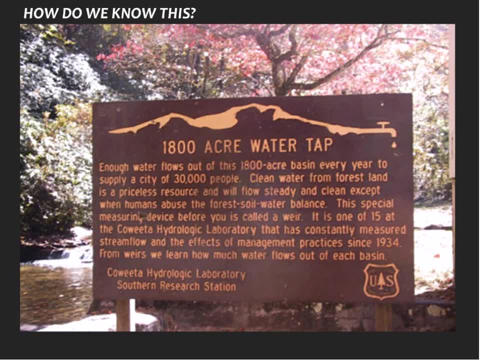 This is a good thing. It's a good thing. This is a good thing. It's a good thing. It's a good thing. It's a good thing, And those experimental forests and watersheds have provided a tremendous amount of information. 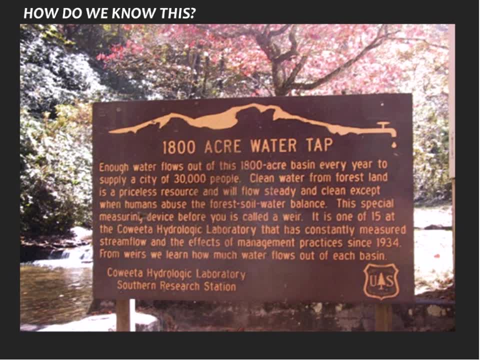 a tremendous amount of sound science on the relationships between forest water. The graphic that you see on this slide is where I spent the first 25 years of my career and where I developed a lot of the information that I'll be presenting today, So I will primarily be using Resolver. 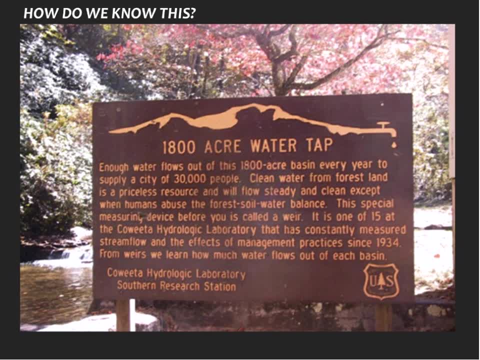 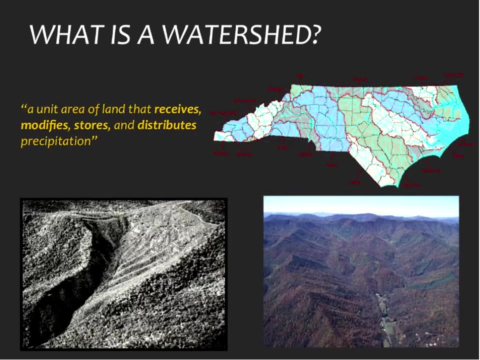 results from studies that are on or around the Cow Wheat Hydrologic Lab, or certainly in the southern region, But the principles that I'll talk about will be generally applicable across the entire United States and certainly in the eastern United States. So let's just start with the simplest notion, and that is what's a watershed. 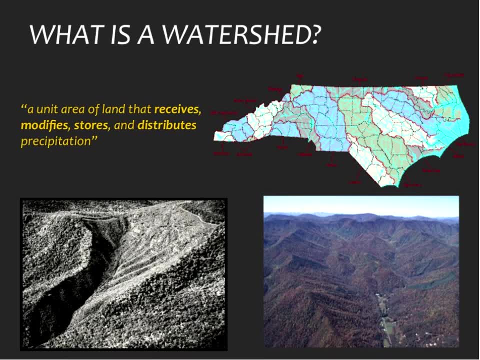 And quite simply, a watershed is a unit of land that receives, modifies, stores and distributes precipitation. They can be small. They can be large, ranging from the small, say 50-acre watershed that you see in the black and white photo on the left, to a 6,000-acre basin on the color photo to the right, to large. 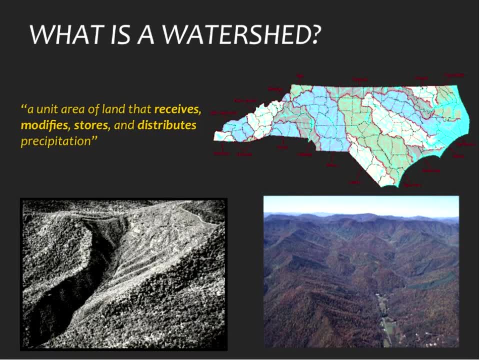 river basins in the state of North Carolina on the upper right. Now, the easiest thing to understand and where most of the studies have occurred are in these small headwater watersheds, And part of the reason is because you can control many of the complexities. 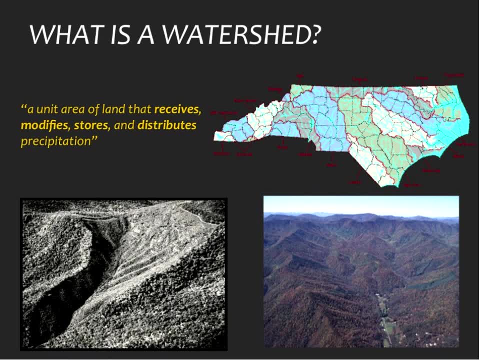 Watersheds are essentially the same vegetation, the same aspect, et cetera. As you move from that small headwater scale watershed to larger and larger scales and up to landscapes, it becomes incredibly complex And instead of the watershed being comprised of one land cover type, it now becomes a watershed. 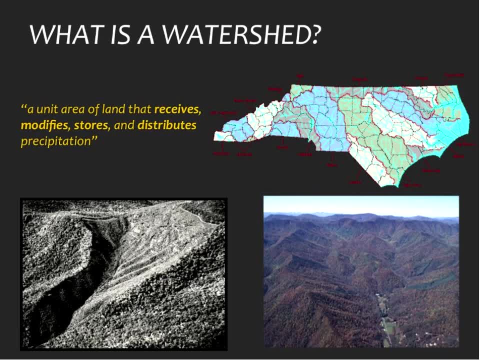 comprised of urban, suburban agriculture, forests, in a diverse and interconnected matrix, And I encourage you to join the webinar in a month or so which talks about the implications of some of those complexities at those larger landscape scales. What I'm going to focus on primarily today, however, is the scale in the lower left-hand. 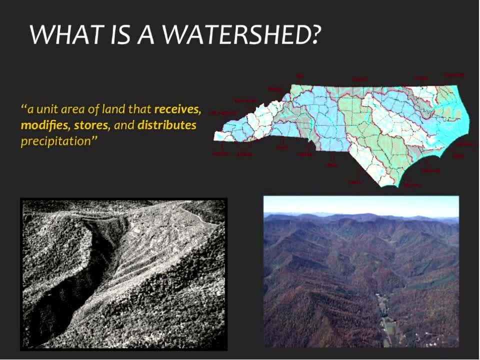 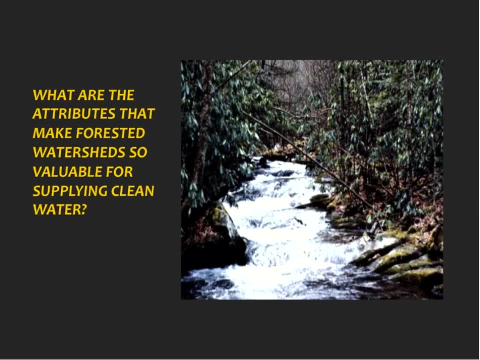 corner, essentially the small watershed comprised primarily of forest cover. So what are the attributes that make forested watersheds so valuable for supplying clean water? And what I want to do is just kind of review in a general way what these key attributes are and then tie those into how those might be changed or manipulated by management activities. 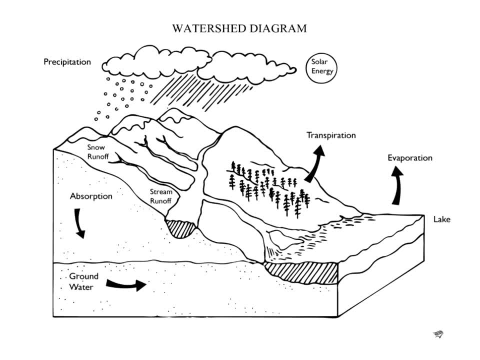 Well, in its simplest form, this is a watershed diagram. This is a large example of a large watershed where we have the inputs and precipitation, outputs and transpiration. what's left over ends up going into the streams or going into the ground. 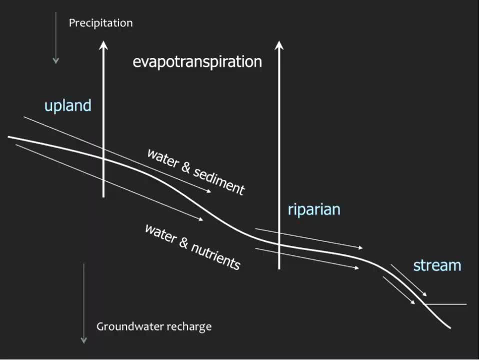 Water for groundwater recharge. But what I really want to focus on is sort of the internal processes that go on within a watershed that ultimately regulate the quantity and quality of water. Same kind of model as before, in that we've got precipitation inputs and evapotranspiration. 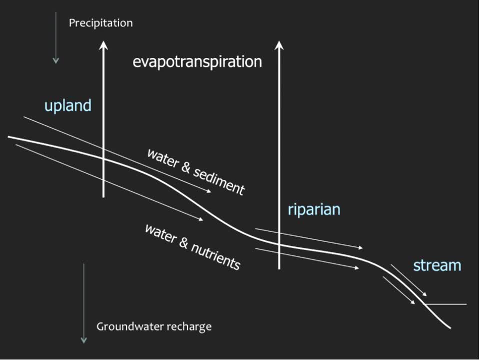 outputs, but how that residual water, or how that water that's left over after there's an evapotranspiration loss, moves across the watershed is a strong regulator of both water quality but also the quantity and timing of stream flow. What flows across the surface is important for delivering sediment to the stream, and 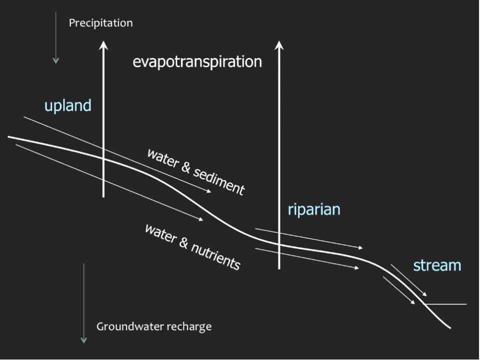 also has a strong impact on storm flow patterns. What flows beneath the surface is important for delivering nutrients and also has an important role in generating base flow and mitigating some of those extremes that might occur That might occur from high intensity storms. Also, note on this graph that I have distinguished the upland forest from the riparian, because 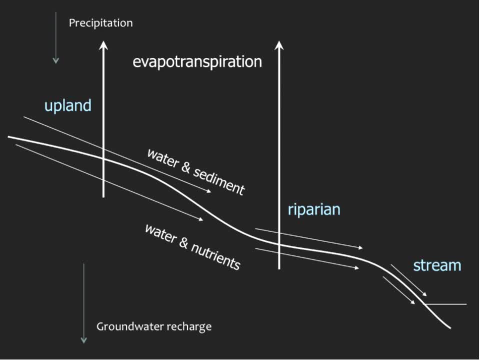 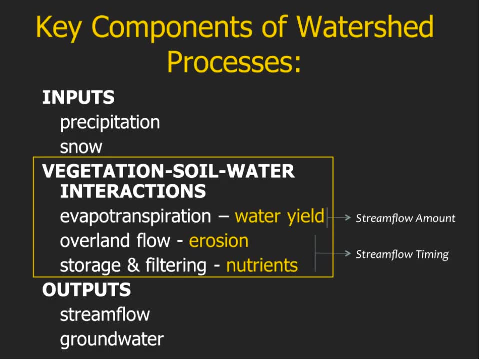 the riparian area has a very critical role in moderating especially water quality but to some extent water quantity, And I'll discuss all of these attributes at some point here in the presentation. So I'm going to really just focus in on the attributes that are in this box. 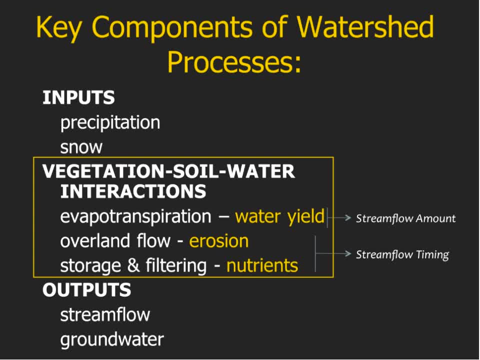 I'm going to talk primarily about vegetation, soil, water interactions, How those are influenced by evapotranspiration, overland flow, and storage and filtering. Although the type and distribution of precipitation and snowfall is important, I'm not going to focus on that much here in the presentation and I'm not going to focus much on the outputs. 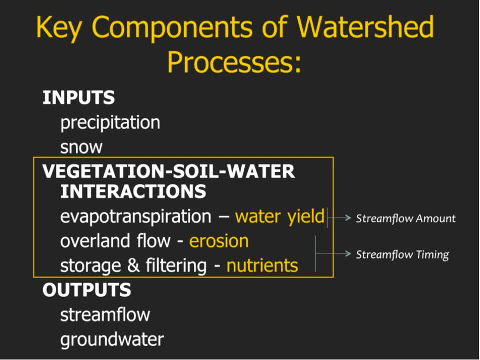 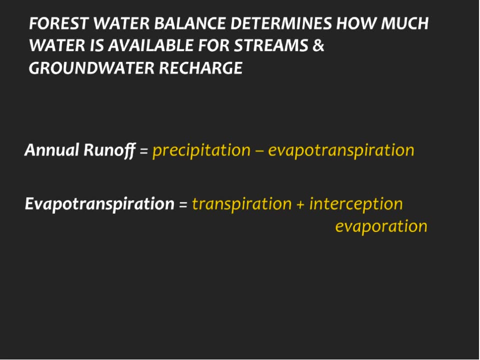 in terms of things like storm flow or groundwater recharge. I'm primarily going to focus on those key watershed processes that determine water quantity and water quality. So, ultimately, what determines how much water comes off in either surface runoff or how much comes off in terms of being able to recharge deep groundwater, is determined by 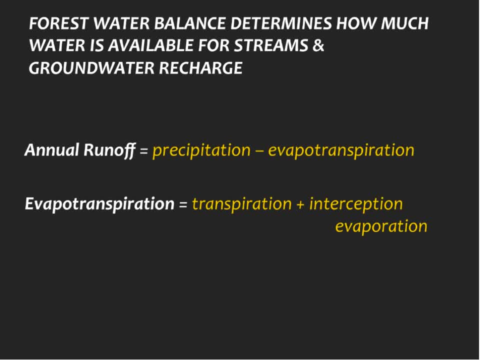 the balance of the forest water balance. And that is essentially, in its simplest form, the difference between how much comes in precipitation and how much is lost in evapotranspiration. Evapotranspiration is comprised of two components. transpiration: how much is taken up by the 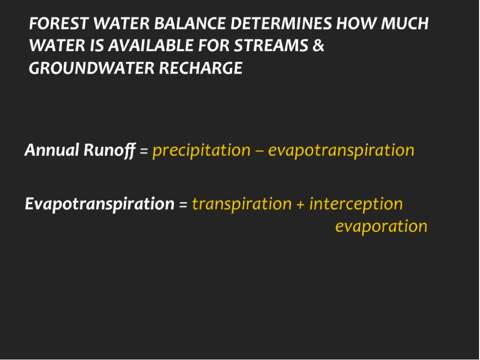 trees and lost through the stomata and interception evaporation. Now this can be a. this evapotranspiration component can be a tremendous amount of the water budget In areas where stream flow is really low and variable and in some cases have very little. 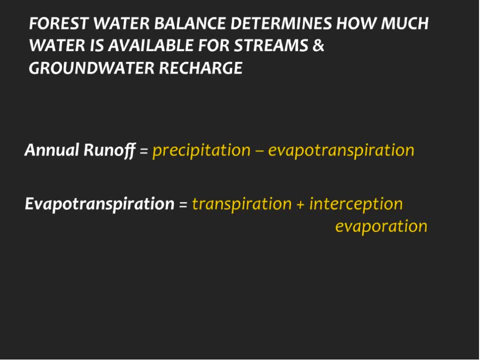 base flow or perennial flow. Usually that's a situation where evapotranspiration doesn't have a lot of base flow. That's a situation where evapotranspiration doesn't have a lot of base flow, So the evapotranspiration and precipitation are essentially equal or, in some cases, potential. 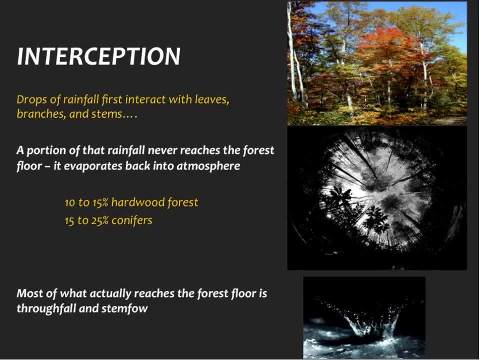 evapotranspiration is even greater than precipitation. So let's first talk about interception. A raindrop very rarely makes it directly to the forest floor. on a forested watershed, A portion of that rainfall actually never reaches the forest floor and it's evaporated. 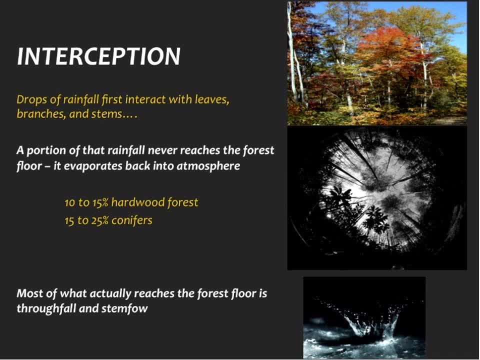 back into the atmosphere. In hardwood forests that value ranges from about 10 to 15 percent. In aquifers it ranges from about 15 to 25 percent. Now, this is an interesting phenomena and a lot of people don't realize it. that up to 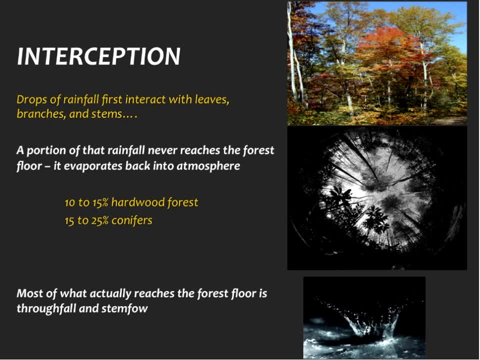 25 percent of the rainfall that falls on a forested watershed never actually makes it to the ground. It's intercepted and evaporated back into the atmosphere, And that higher number occurs when you have annual rainfall, where you have a lot of light rain, or whether there's a significant amount of leaf area or branch branches that intercept. 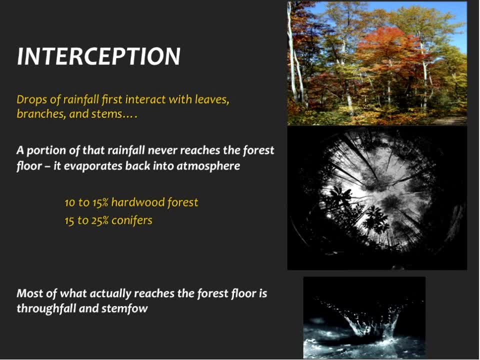 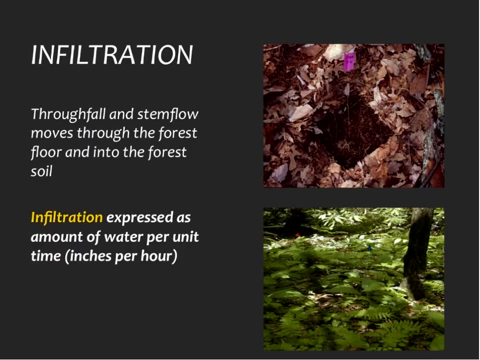 and provide that surface to evaporate back out. So most of what actually reaches the forest floor is through fallen stem flow, and that's anywhere between 90 to 75 percent of what comes in precipitation. What then does come through through fallen stem flow moves through the forest floor through. 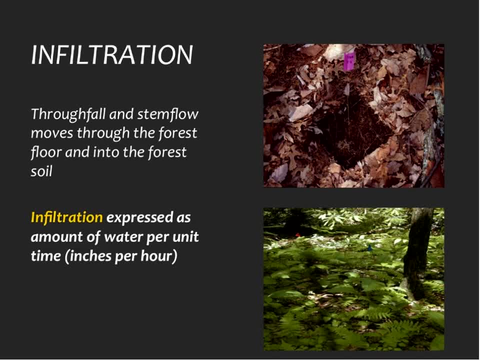 the process of infiltration And you can see from these figures what really distinguishes a forested watershed from a forested watershed from most other land uses is two things. One is, in some ecosystems, a fairly dense understory vegetation, which is shown in the lower graph. 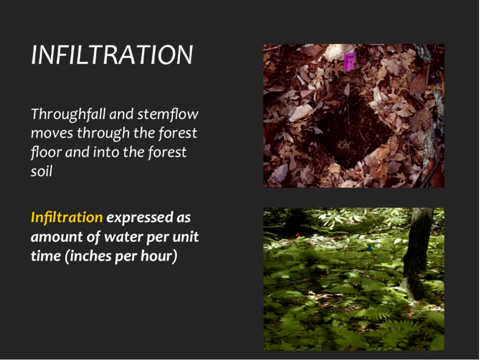 which adds another barrier and another place where you can get some interception and evaporation, But also a very thick forest layer, litter layer and humus layer. So, again, very rarely does a raindrop that comes through an infiltration directly hit the soil. It has to pass through another round of vegetation in the understory or through the thick layer. 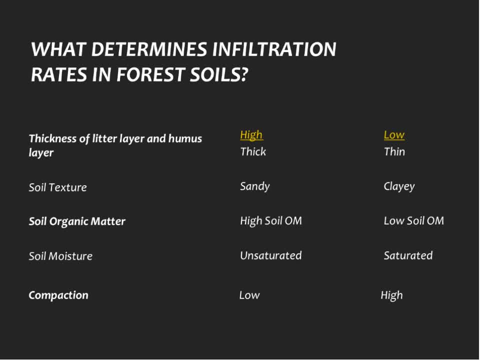 litter and humus layer. Now there's lots of things that determine infiltration rate. Some of them are physical, which and essentially uncontrolled by forest management activities, and that would be things like soil texture. There's not much that can be done about soil texture. either have a sandy soil or a clay. 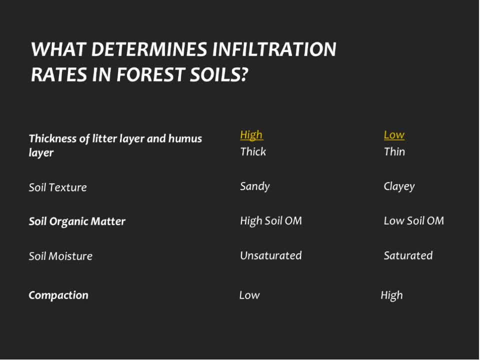 soil or silt loam. But there are other things that are more biological in nature and can be impacted by forest management activities, such as the thickness of the litter layer, the amount of soil organic matter and the level of compaction. The kinds of conditions that promote a rapid infiltration rate would be a thick litter. 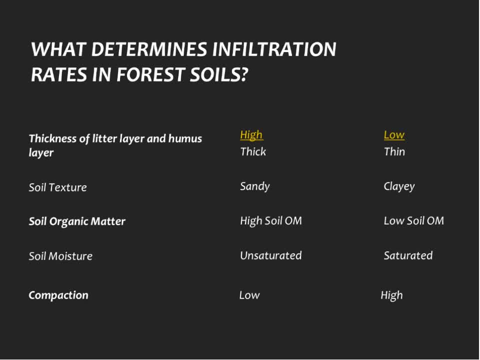 layer. a coarse textured soil like sandy soil, high soil organic matter, unsaturated antecedent conditions And low compaction And the kinds of things that would precipitate low infiltration rate would be a thin layer. clay soils, low soil organic matter, saturated soil, such as after a heavy rain or in areas. 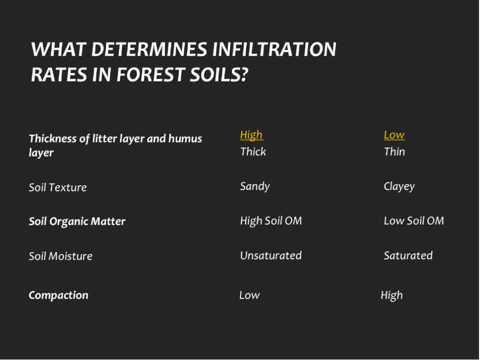 that have a high water table or areas that have been highly compacted, And you can begin to see that if you do have a situation where you have a very clay soil characteristics that you can control, like a thick litter layer or high soil organic matter or reducing compaction could be important. 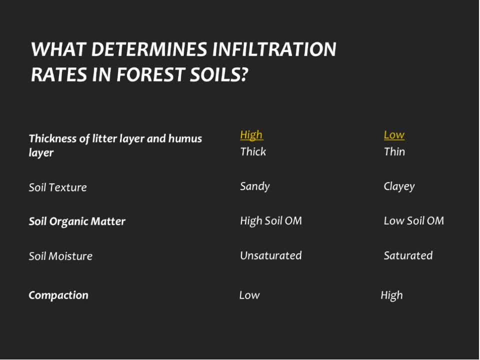 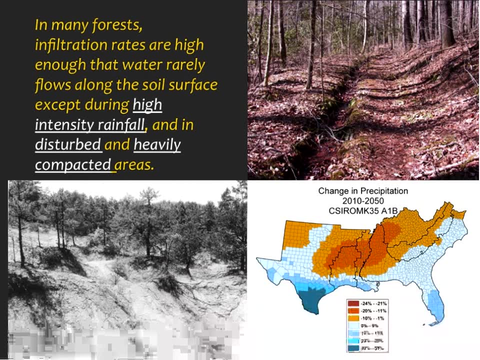 So that's one of the things that we're going to talk about in a little bit. Thank you, That's very important for offsetting that low infiltration rate. For the most part, overland flow, or hortonian flow as it's called, doesn't happen very often. 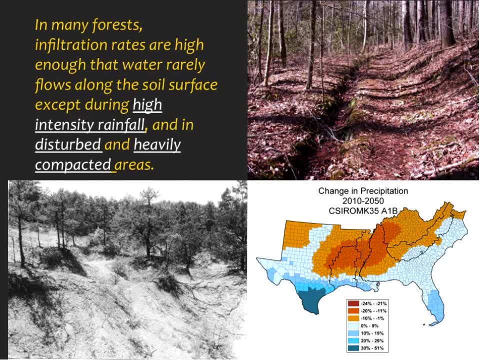 in many forests because the infiltration rates are really high, or certainly high enough that water rarely flows along the soil surface. Now, there are exceptions to this, and there are certainly times where rainfall intensities are so high that There's a lot of water that flows along the soil surface. 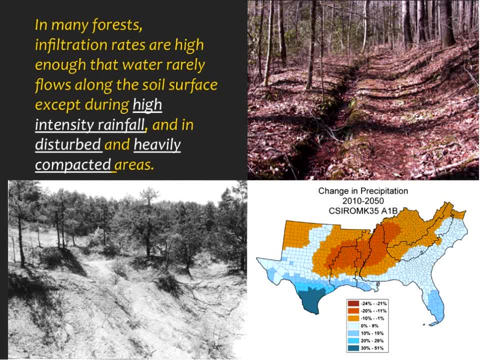 that water and you know, especially if it's a long, high-intensity storm, that all the pores in the soil get filled up and water can flow along the surface. but it also can happen in heavily disturbed or heavily compacted areas as well, and these graphs kind of show in some of the worst case scenarios down the lower is. 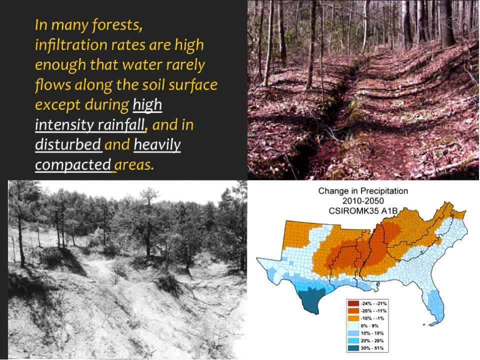 some historically bad land uses in the southern United States that have very high erosion rates, very low infiltration rates, and then the upper right corner is a classic example of an abandoned legacy road where that long-term compaction essentially allows water to flow right down the middle and sort of a mini. 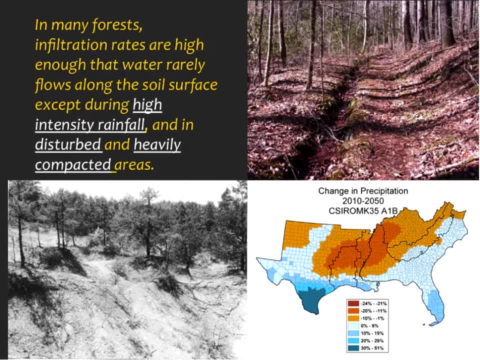 stream and then the lower right hand corner is is to discuss a little bit about what might be to come in terms of infiltration rates. is that, if there is a continuation of increased frequency of severe storms and high-intensity rainfall events with, with climate change, the notion of overland flow and erosion, and 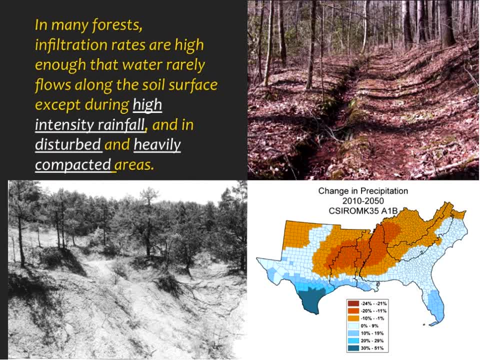 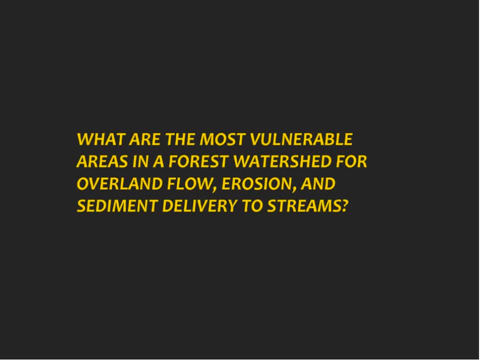 sedimentation may come with. that may become an increasingly important factor for land managers to deal with. so first question, just to get a little bit of participation by the audience here. there is not an ABC or the answer here. this is one where I'll give the answer in the next slide, but the first first. 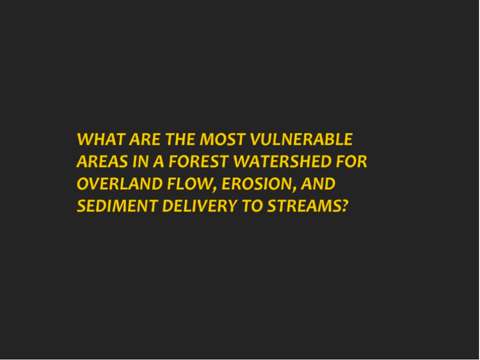 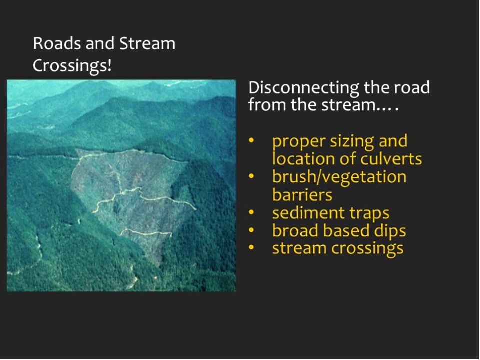 question to think about is is based on what you know and what I've told you so far. what are the most vulnerable areas in a forest watershed for overland flow erosion and sediment delivery to streams? think about that for a minute and then I'll click on the next slide. okay, and Jim, if people would like to answer in their 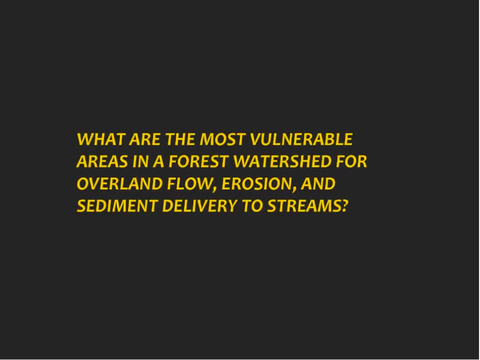 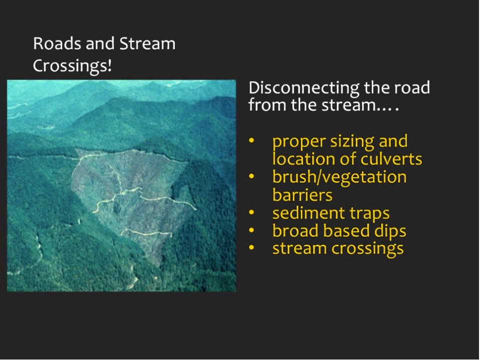 chat box to: okay, welcome to use that to begin some discussion on the answers and, okay, any questions that you've had to date. okay, thank you. well, I kind of gave away the answer, but one, one of the early, early questions that cow eaters and and a. 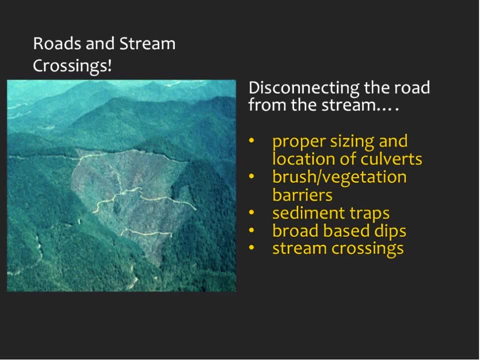 lot of experimental forces is what causes erosion, in combination with with force cutting- and many believe that it was this- the mere act of cutting the, the forest themselves was a cause of erosion- and what the science has shown? that the real critical areas for erosion and sedimentation are the roads and the stream crossing in watersheds. 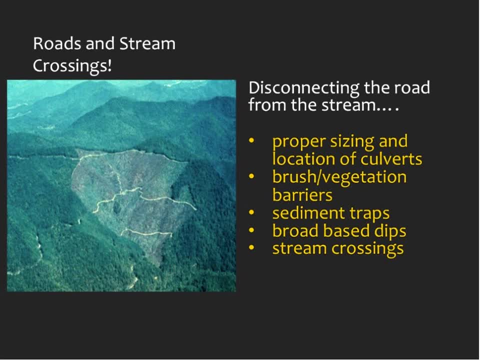 And so best management practices that protect or disconnect the road from the stream through proper size and location of culverts, proper and complete brush and vegetation barriers, things like sediment traps, broad base dips and close attention to stream crossings are really critical for disconnecting the road from the stream. 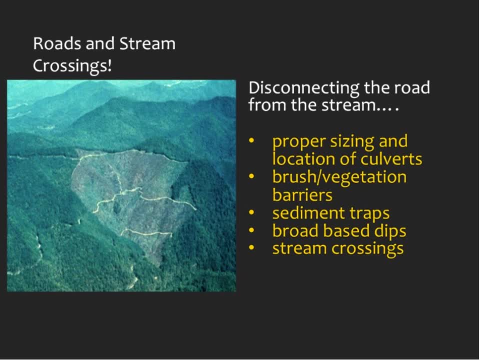 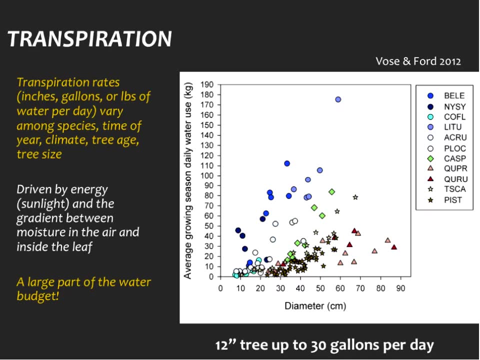 Again. you'll learn more about this if you tune in again, I think in the third webinar on best management practices and water quality. Another large component of the water budget is transpiration, So we talked about interception. water drips down through the forest canopy and stems. 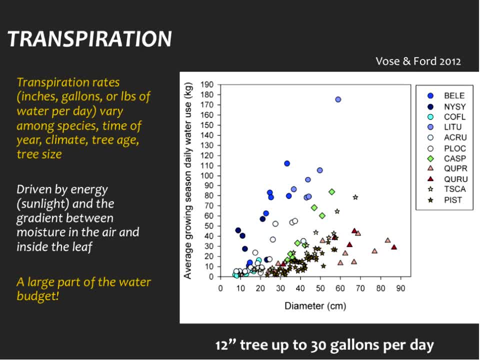 It infiltrates into the soil. Now some of that water, then in some cases a large amount of that water is going to be used by the trees. Transpiration rates can be a very large part of the water budget, sometimes up to 80 percent. 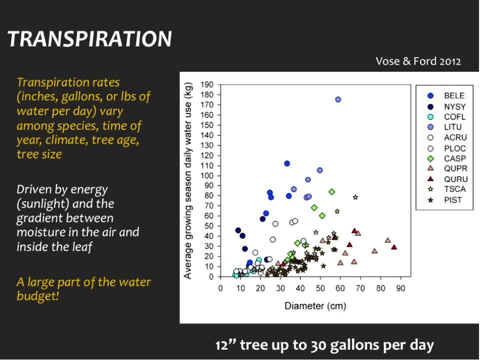 in some environments 100 percent of the water budget. So this is a big part of the water budget which can be manipulated, either intentionally or unintentionally by management choices. The rates vary among species, Vary among time of year, climate and tree age. 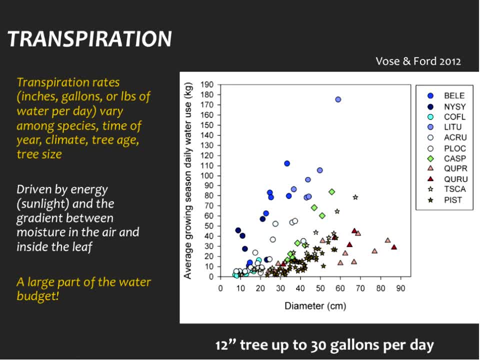 And this is driven by the gradient right, by energy and the gradient between the moisture in the air and the inside of the leaf through the stomata. The graph on the right hand side are some, actually some pretty rare data With the advent of some technology, scientific measurement technology called sap flow scientists 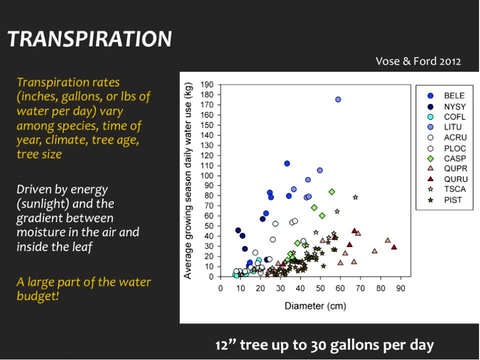 are now beginning to be able to individually estimate, Okay, How much water certain tree species use. On the right hand side you see the color codes of a bunch of different species. If you remember some of your Latin names of your trees, you'll recognize these, or might. 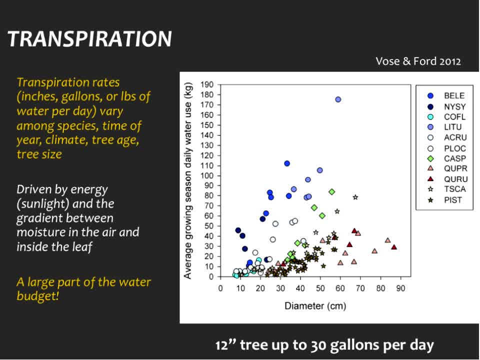 be able to guess them, But I'll just run through them. There's Betula lenta or birch, Anissa sylvatica, black gum. Cornus florida, dogwood. Liriodendron tulipifera is yellow poplar. Acer rubrum is red maple. 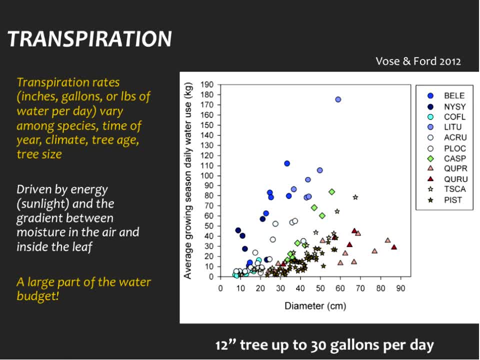 Looks like there's a Platinus ocidentalis which is, I think, a Sycamore. There's a Hickory Caryus species, a Quercus prinus, a chestnut oak. Quercus rubra red. 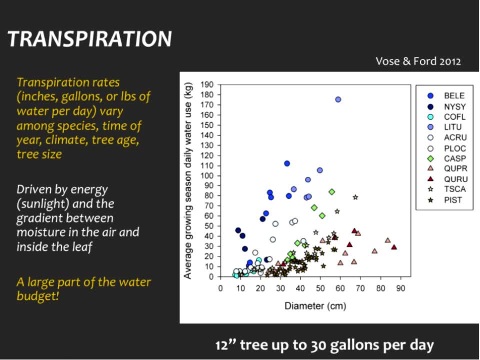 oak Hemlock pseudocanadensis and white pine Pinostrobus. What you'll notice is, let's just say, at 30 inches of diameter, which is about a 12-inch tree. the range and the amount of water used by these various species varies from about 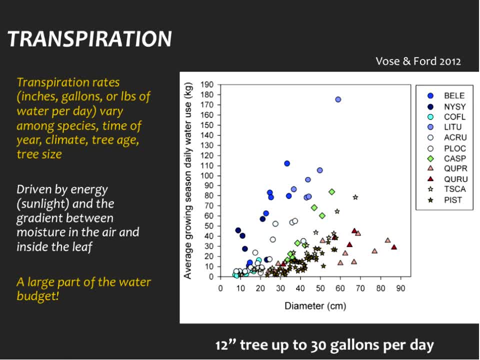 10,000 feet to 3,000 feet. Okay, kilograms per day to 100 kilograms per day. so huge variation in the amount of water that individual species can use and that has a lot to do with its morphology, physiology, xylem, anatomy, The 12-inch tree, just to put it in units. 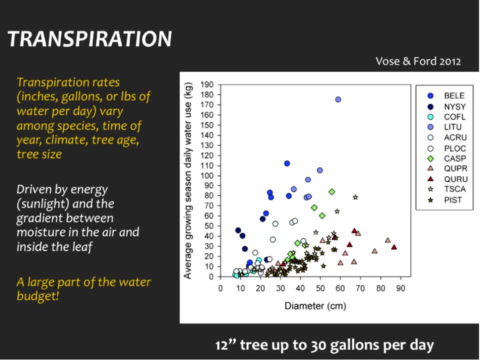 that might be more familiar with you, a 12-inch tree, and this, using these data, is using up to about 30 gallons of water per day. So you can see that, depending upon the successional stage, which might favor one species over another or 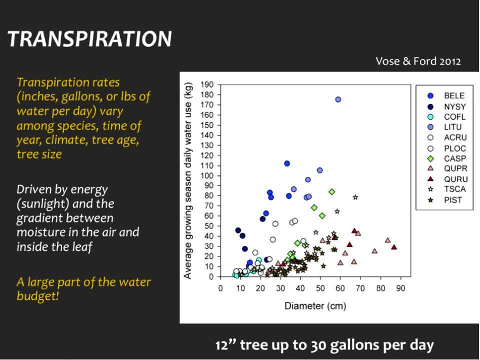 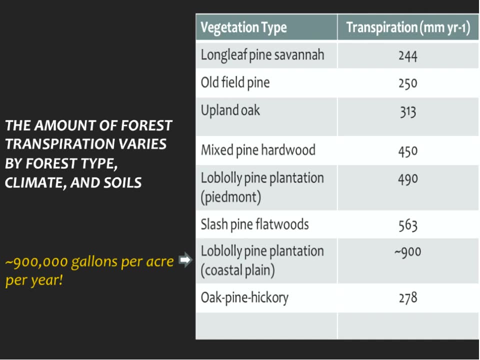 management choices which favor one species over another, there can be a very large difference in the amount of water that's transpired by the particular species in the forested watershed, And this then begins to translate into forest types, which are comprised of predominant species types. 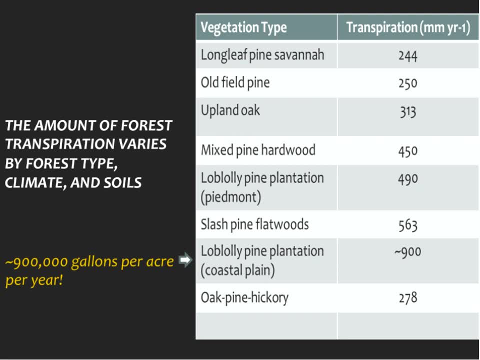 So the amount of water that's transpired in the forested watershed can be the amount of water that's transpired in the forested watershed. So the amount of of forest transpiration varies by forest type and is influenced by the climate and soils where they grow. In this case, the the box on the right-hand. 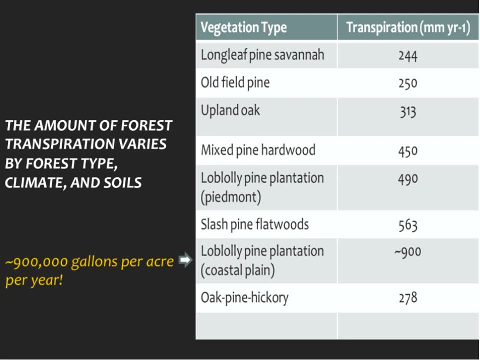 side there shows a range of about 244 millimeters per year of transpiration longleaf pine savanna upwards to about 900 millimeters per year in transpiration in a low lavalier pine coastal plain forest, sitting in essentially a bathtub of water. So very large differences in the amount of water. 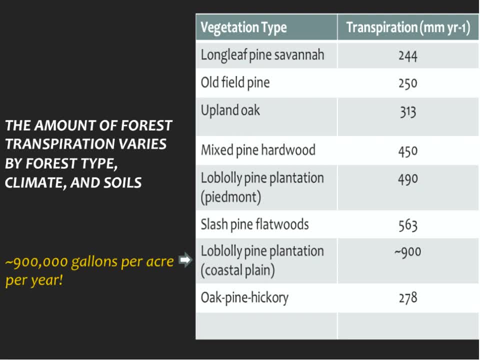 that is used by these different forest types and if you use that water balance, that precipitation minus evapotranspiration, the result would be very large differences in the amount of stream flow coming out of these forest types, or a lot of differences in the amount of groundwater recharge capable. 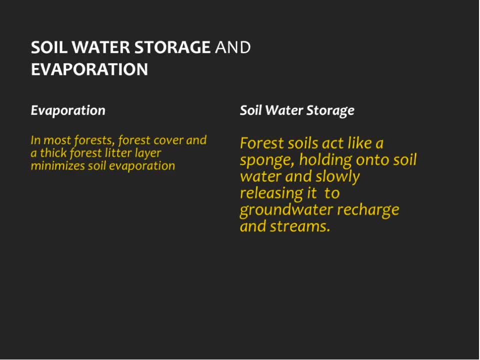 from these forest types. Now, the water that's not used by transpiration, then is essentially either evaporated out through the forest floor. That is a very low amount in most forests because the forest cover and thick forest litter layer minimizes soil evaporation. But what is a really important process in forests is the soil. 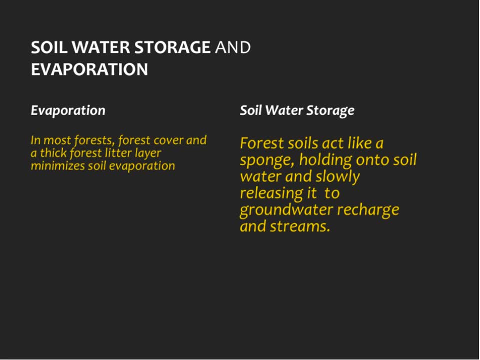 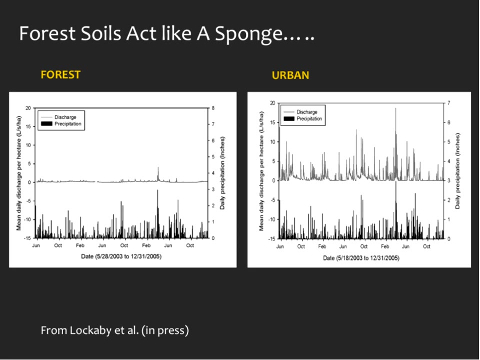 water storage component, and the analogy is that the forest soils act like a sponge, holding onto the soil water and slowly releasing it to groundwater recharge in streams, And this process is really what's going on in these two graphs that I show here. These are two side-by-side watersheds receiving essentially the same amount, or 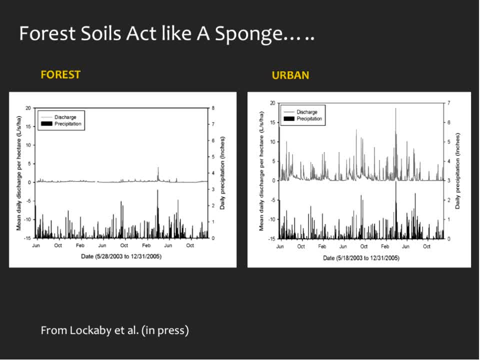 the same pattern of precipitation. The one on the left with the title forest is a forested watershed. precipitation are the black bars. discharge and stream flow is the gray line with the very small bars On the right side is the same units: precipitation子all use glioblast. discussion is clean water? 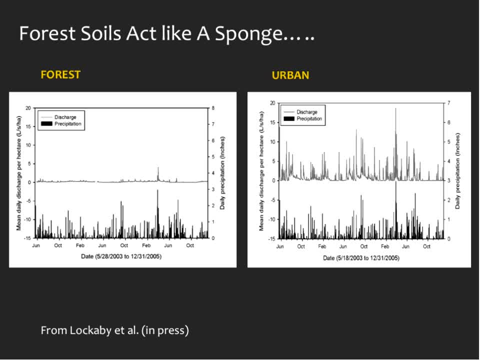 in the black bars, discharge in the gray bars And you can see a very large difference in both the amount of water that's coming out of the watersheds and, more importantly, the pattern. The one on the right side has much higher flows but a very spiky pattern that almost 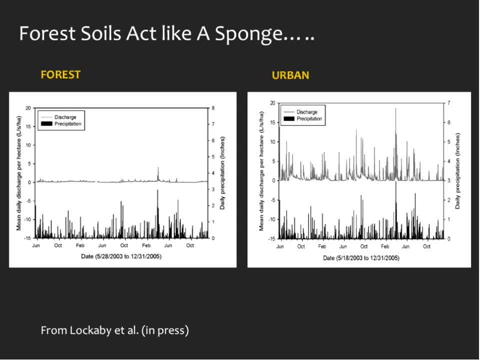 mimics the precipitation inputs, And that's due to the fact that the large impervious surface results primarily in overland flow and not that soil, that slow water release that comes from that forest soil, acting like a sponge. Now a lot of folks have thought: well, isn't this good that all this extra water is coming? 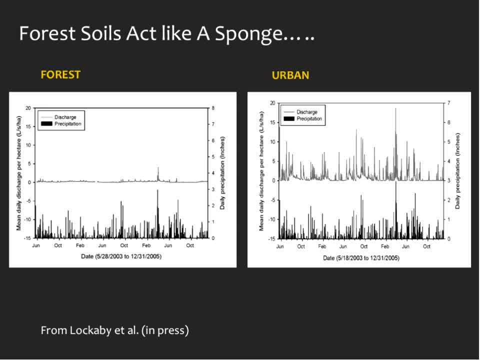 out of this urban area. wouldn't that be a way to solve water supply problems, because there isn't that water use by the trees. Well, a couple of things happen. One is: most of this water can't be captured. It's flowing so fast that it flows right through water treatment facilities or flows right. 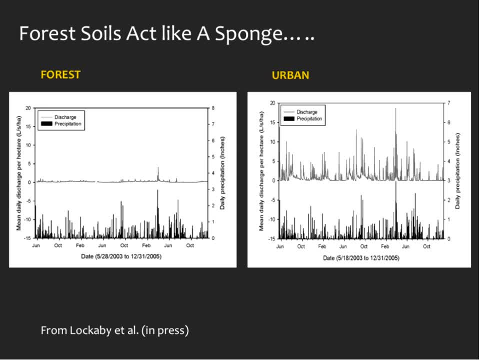 over or right through storage reservoirs, and it doesn't recharge groundwater. The second thing that happens is that, in addition to this water being so fast and delivered in flashes or pulses that it can't be used, it almost always has a much lower water quality. 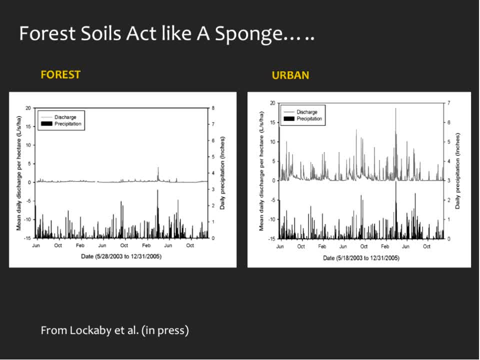 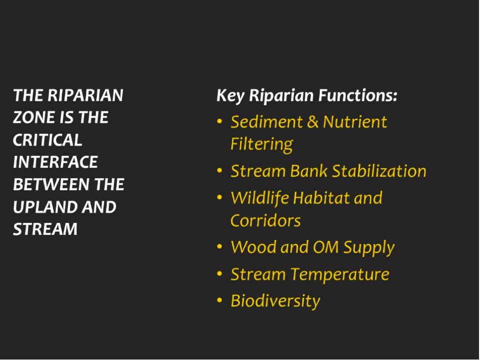 as well. So any gain that might be achieved for the extra quantity is offset by the reduction in water. Okay, so what I'd like to do now is just hone in on one of the key zones in a watershed, and that's the riparian zone. 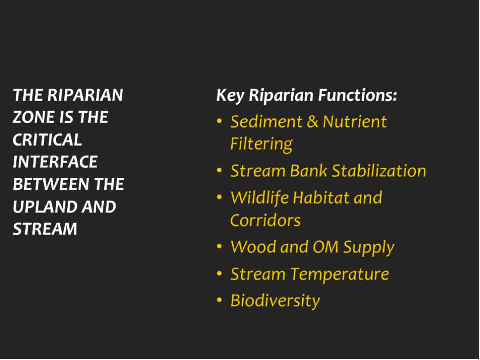 And that riparian zone is a critical interface between that upland component of the watershed and the stream. Now you have a riparian zone whether you're in a flat area without a lot of topography, or whether you're in a very steep mountain watershed. 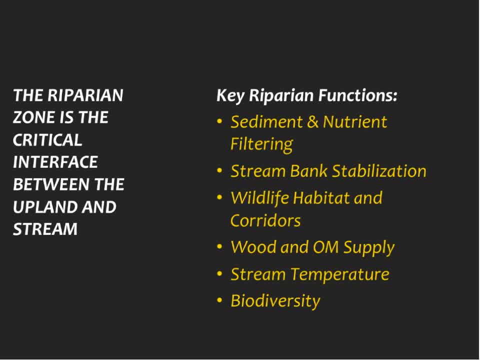 All watersheds have that a riparian zone in that near stream area And of course the riparian zone has some key functions. Most of you know these: sediment nutrient filtering, stream bank stabilization, wildlife habitat corridors, wood and organic matter supply, stream temperature, biodiversity. 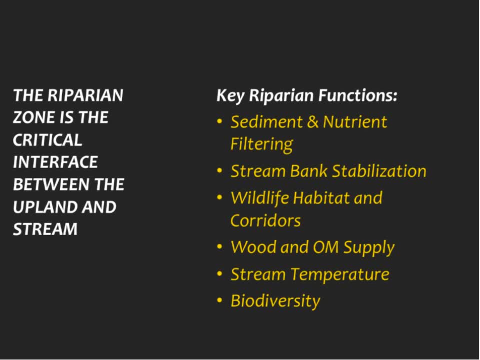 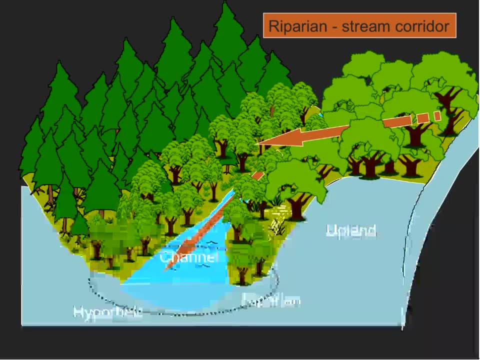 The primary function, though, that I'm going to talk about is the first one, and that's the sediment and nutrient filtering function. Okay, Okay. So when that water moves down through gravitational forces, down from the upland down into the riparian zone, there's really two areas of interaction. 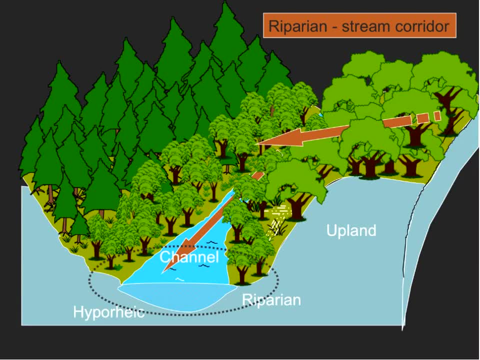 One is in that hypereric zone which is the subsurface interaction, where primarily nutrients are exchanged back and forth. That's the one that's in the dashed circle there. And then the other area of interaction is what flows down through lateral flow, Down through the unsaturated or in some cases saturated soil from the upland. 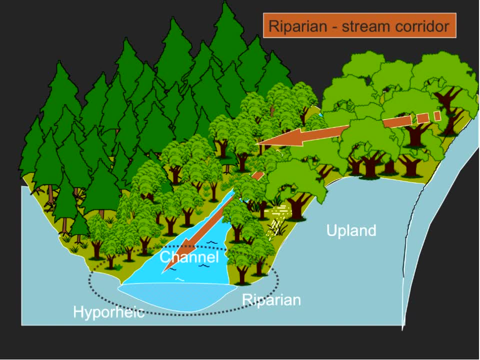 And that, of course, is also exchanging nutrients and water. And then if there is going to be any overland flow, it typically might occur in that riparian zone where it's more likely that the soil will be surface, will be saturated, So there may be some overland flow, especially during high storm events, in that riparian. 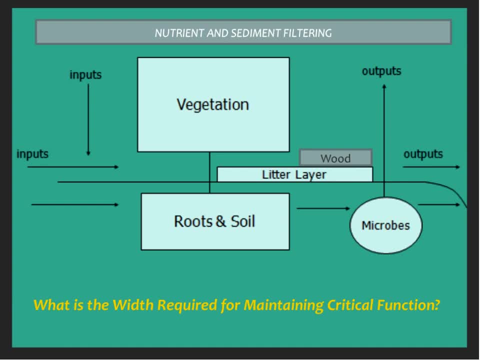 area as well. Okay, Okay, Okay, Okay, Okay. So the 3 processes that are really important in their role for maintaining the ability to filter both sediments and nutrients, The first and foremost is the riparian zone. for it to be functioning effectively, needs 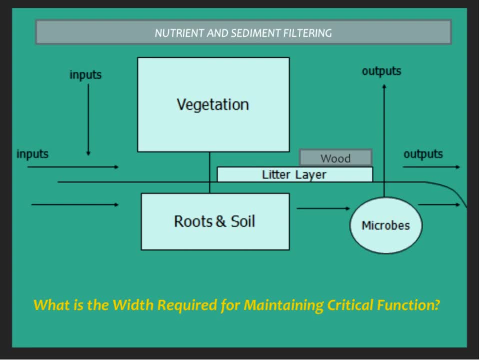 to have vegetation And that vegetation can be, and is typically about above ground. You know, I'm sorry, uh, woody or trees, But also the shrubs and the herbs in that riparian zone are really important for trapping and cycling nutrients that may be flowing through the subsurface. 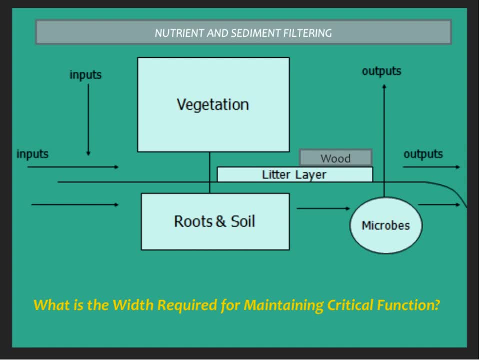 The litter layer in the wood are very important for filtering any of the sediment that flows down- if it does flow down in overland flow, and having a good, coarse woody debris layer in that riparian zone is critical. The other thing that's important is microbial activity. 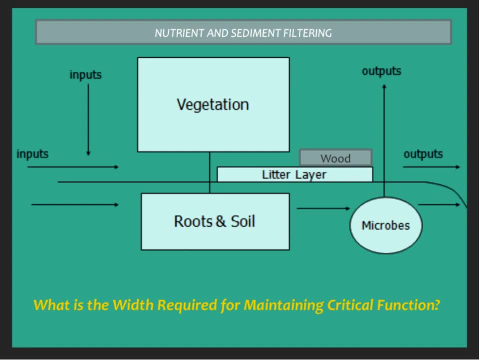 In riparian zones that are frequently wet and in some cases saturated. the microbial activity is really important for either immobilizing nutrients in their normal biological processes or for nitrogen in particular. the process of denitrification is actually a way where organic nitrogen that might, an inorganic nitrogen that would flow into the stream, would. 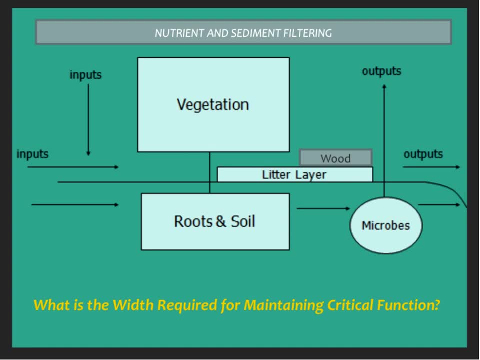 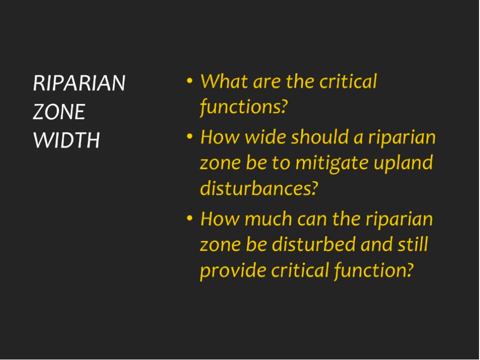 be converted from that elemental phase in the soil solution To a gaseous output which is shown on the right side bubble coming out from the microbes. So very critical functions, some of which are unique to the riparian zone, especially the microbial processing, and doesn't occur in the upland. 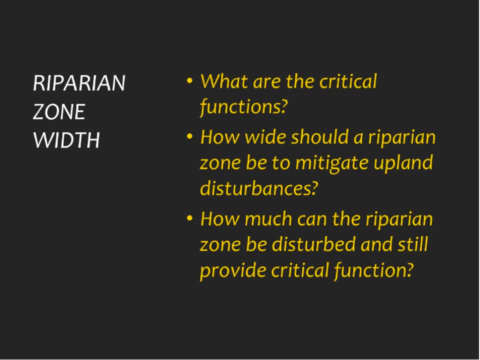 So there are some, and continue to be some, real critical issues related to riparian zones, and one of the most important questions that's asked is: what is the proper riparian zone width in a forested watershed? So the answer to that is yes, It's a good question. 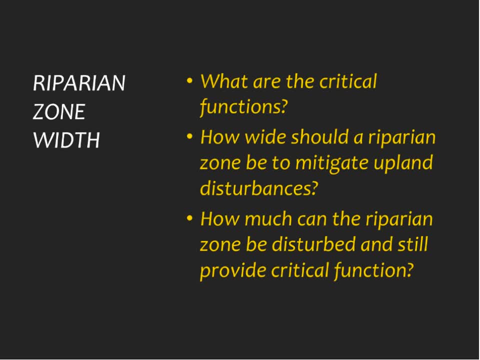 And that can be defined in a variety of ways. but one of the ways it can be defined is: what are the critical functions that occur within whatever that width is from the stream edge towards the upland system? And I'm going to talk about that a little bit here in the following slides. 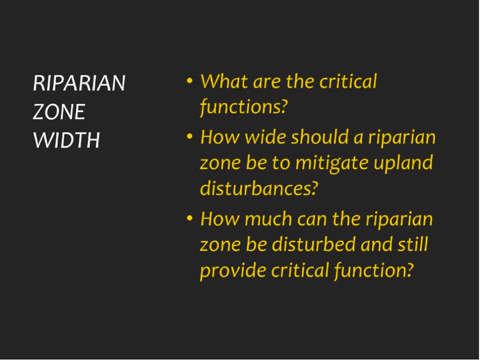 The other questions that are really important and will be talked about in the best management practice webinar- a couple of webinars now- Is: how wide should the riparian be to mitigate upland disturbances And how much of the riparian zone can be disturbed and still provide critical function? 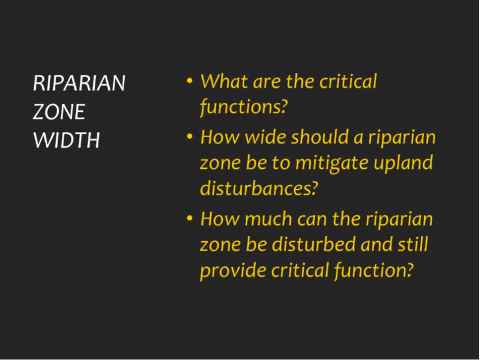 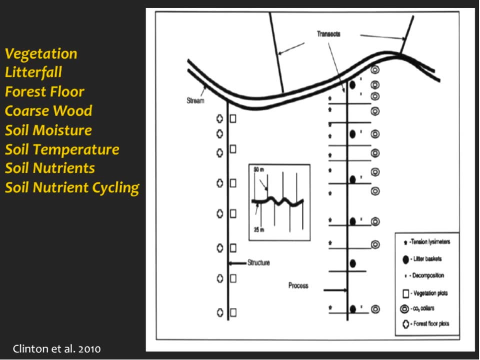 All of these are have a fair amount of science behind them, but still uncertain in some places. Now, one of the things I'd like to share with you is an actual study that we did in the mountains of Western North Carolina To try and understand exactly how wide 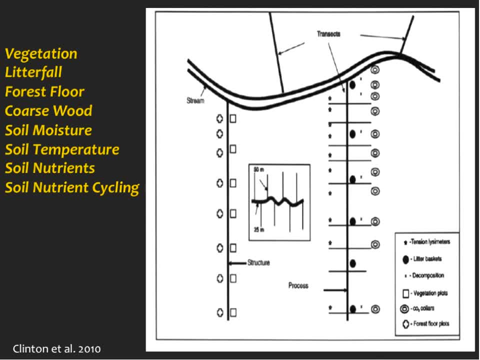 Okay, How wide a riparian zone is in terms of critical function, And these are the types of functions that I showed you in the previous slide, The things that are important for filtering nutrients and sediments. So, how much vegetation is there and what kind is it? 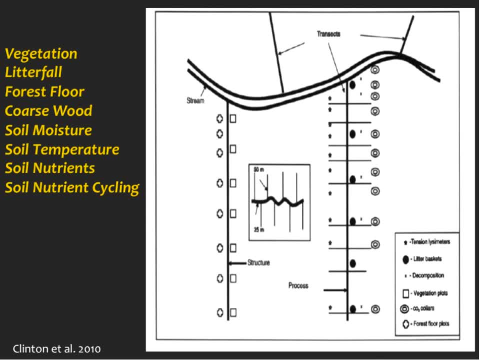 How much litter fall or litter layer in forest floor is there? How much coarse wood is there? What's the soil, moisture and temperature factors that regulate nutrient cycling processes? What are the amount of soil nutrients And how does soil nutrient cycling work? How does soil nutrient cycling change? 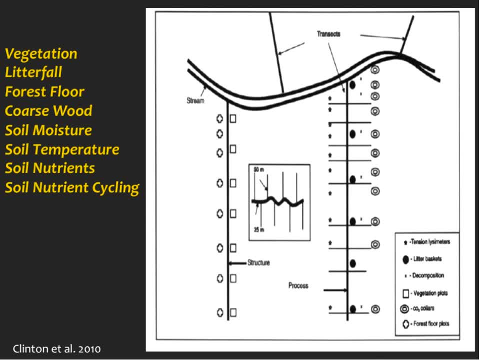 And these are the kinds of studies that need to be done to characterize the width of a riparian zone in a functional way. And essentially what we did is measured these parameters at fixed intervals from stream edge all the way up into the upland forest. 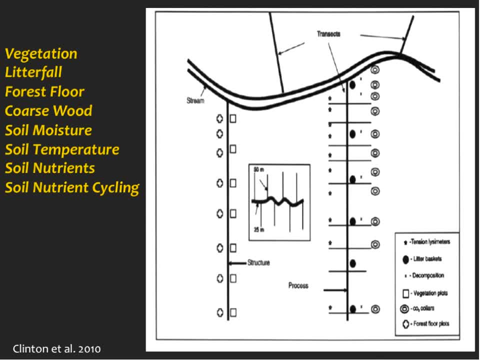 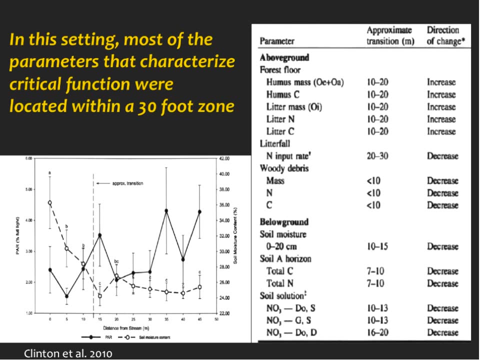 And then looked for where those key parameters changed, With the assumption that where they changed was a reflection of a different functional state. Okay, So this is a transition from riparian to upland forest. Now I'm not going to go into the nitty-gritties of the statistics or exactly how we did it. 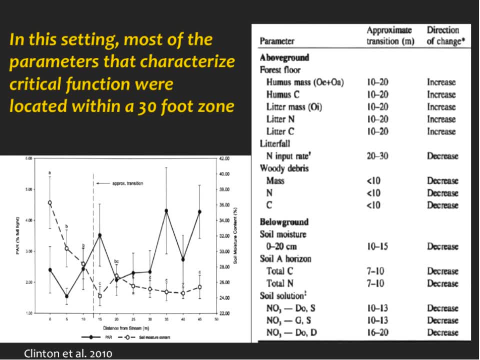 Those data are here and I can send you a paper. You can look up the paper by Barry Clinton in Canadian Journal of Forest Research in 2010.. But basically, what we found is that there was a noticeable transition, a statistically significant transition, in a whole lot of these parameters. 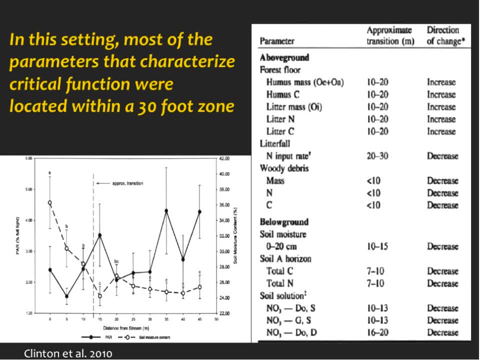 And most of them can be calculated. So what we did is we converged around 30 feet. Now it turns out that the typical riparian zone width in the mountain region, or the minimum width, it was about 30 feet. That was determined basically by experience and to some extent by vegetation characteristics. 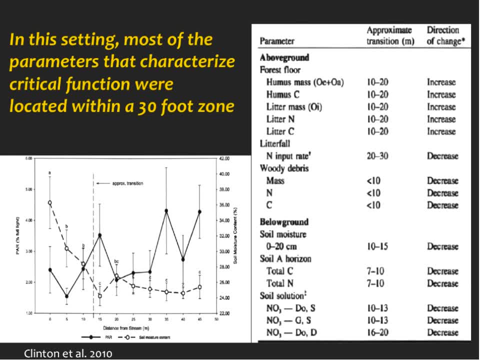 But it was confirmed and shown that it was about a 30-foot riparian's width. So at that area those parameters- Forest floor characteristics, litter, fall, woody debris and below ground soil, environmental and nutrient characteristics- essentially changed So that 30 foot was the functional width. 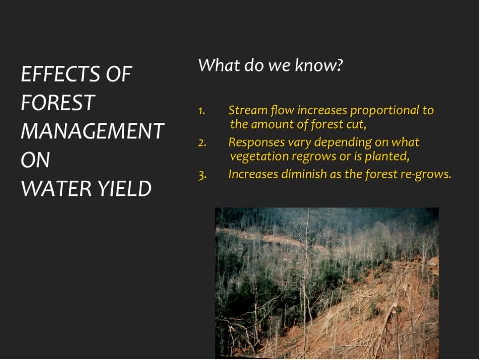 Okay, And again, more will be talked about the riparian zone, best management practices and functional width from a standpoint of protecting from disturbance, and what kind of management activities can be done in them, in a further webinar. Okay, What I'd like to do now, then, is transition into the discussion of sort of an intact forest. 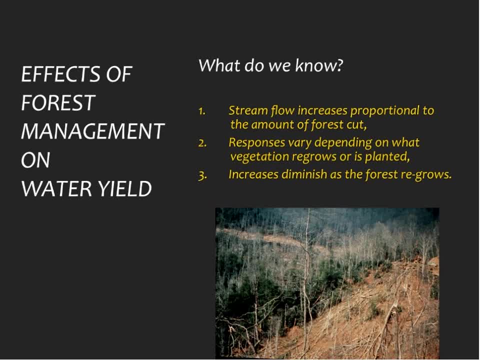 to what happens when the forest is either cut or burned, And this is then titled the effects of forest management on water yield. So I'm going to start with just sort of three statements about what we know, And what we know is that stream flow increases after cutting are proportional to the amount. 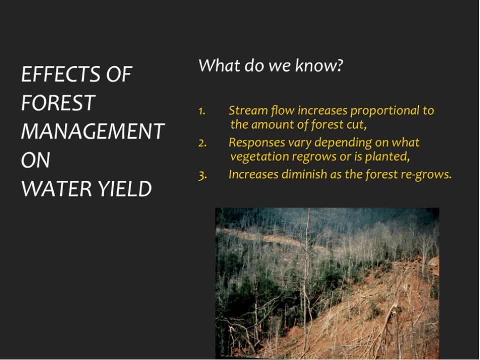 of forest that's cut Now how that responds and how long it responds depends on what vegetation regrows or what is planted behind it, and that the responses are dynamic and that the earliest responses right after cutting diminish as the forest regrows. 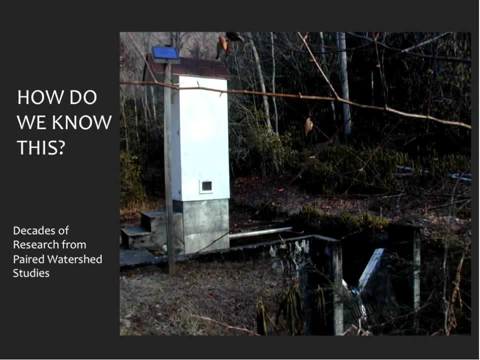 And we know this from long-term- and I mean 60,, 70-year-old studies, So decades of research from paired watershed studies, not only in the south, which is where I'll use as examples, but from watersheds all over the continental and as well as Puerto. 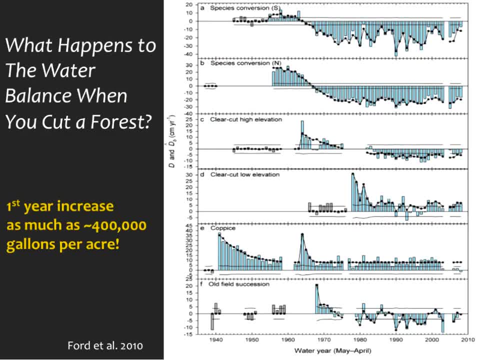 Rico and Alaska, so all over the United States. And so what happens after, or what happens to the water balance when a forest is cut? This graph shows six different examples from these long-term studies. The time stamp on the bottom goes from about 1940 to almost 2000.. 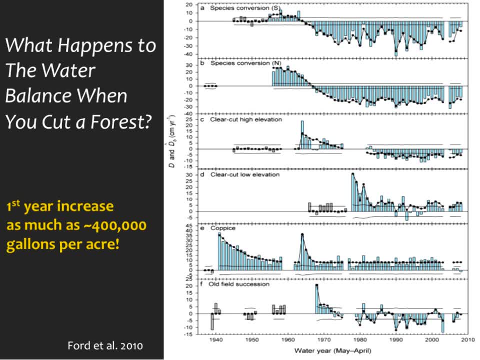 Okay, And this shows how stream flow or how the water balance has changed as a result of cutting and then changes in forest composition after cutting. Now, just to give you some idea of how to interpret this graph: anywhere where you see a zero in the panels, that's no response. 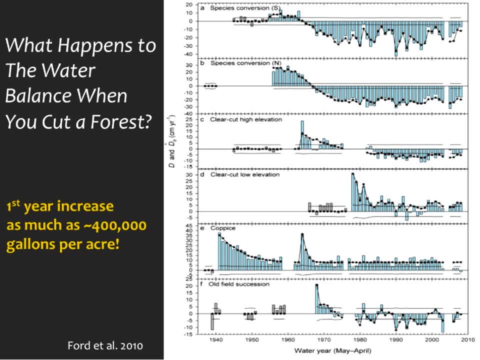 What that means is that the flow of the forest that was cut is identical to the flow of the forest that wasn't cut. Okay, If the value is above that line. okay. in this case, we're talking about the blue bars and the black dots that are modeled to fit the bars, then stream flow from the cut forest. 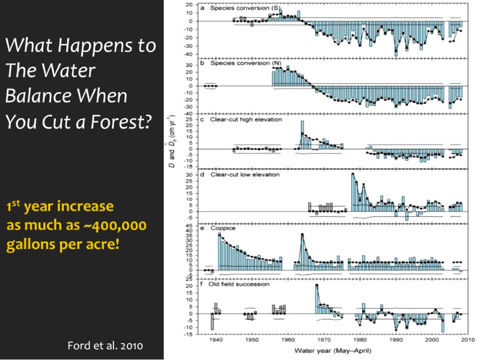 is greater than the reference forest. When the blue bars are below the line, stream flow is less than what happened or what was going on in the reference uncut forest. So one of the first things we note is that stream flow increases. in some cases increases. 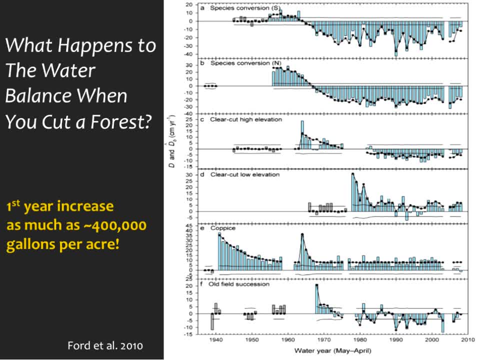 quite significantly When the forest is cut And that's due to removing the leaf, transpiration, surface area and interception, And in some cases the increase can be as much as 400,000 gallons per acre. As the forest regrows, that amount of increases diminishes. 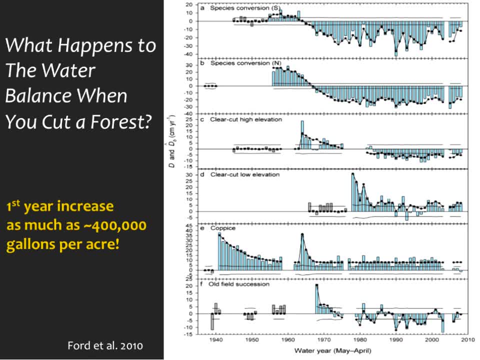 And if we just focus on the upper two graphs, A and B, it essentially reaches the zero point at about in those forests, at about age 15 or so. Okay, Now, the upper two graphs also show that what happens over the long term is that forest. 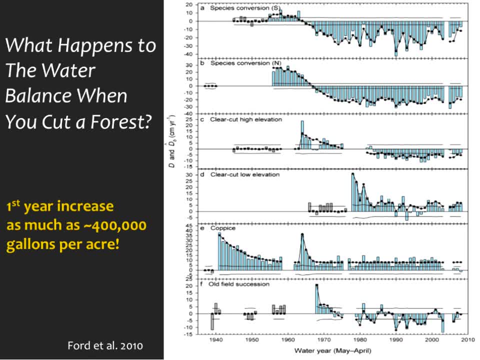 flow, or stream flow, is now much lower than the reference forest than it was before, And the reason for that is that both of these represent an example where the hardwood forest was converted to a pine forest, So the pine forest is using more water than the hardwood forest. 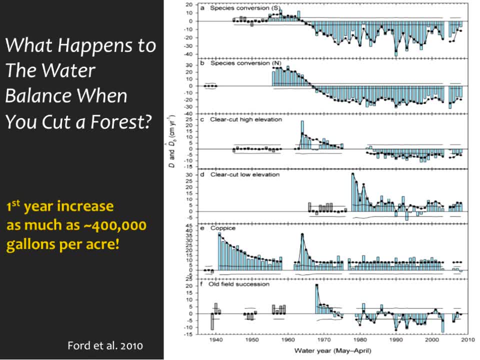 And remember. one of the things that I showed in the graph is that there's greater interception In the pine forest, And that's one of the reasons, And then the other reason is that there's greater transpiration that occurs in the milder. 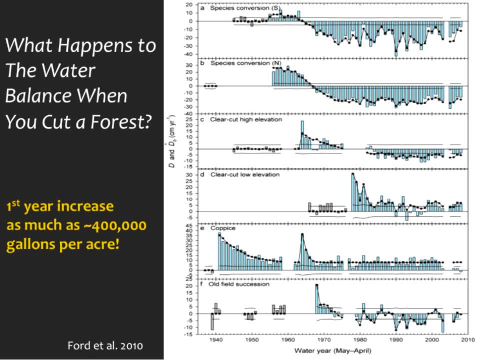 climate here in the southern United States. So this is an example where you get an initial increase in flow. That flow diminishes quickly as the forest recovers to about what it was in the reference forest by about age 15.. And then hereafter flow is about 20 or 25 percent lower than it is in the reference. 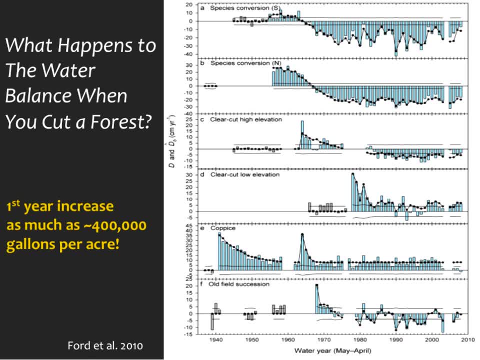 forest That is in the pine. So a shift in that water balance is a result of species composition changes. The other graphs show a variety of other things happening. One is a high elevation clear cut at C: A low elevation clear cut is D, Almost a different. 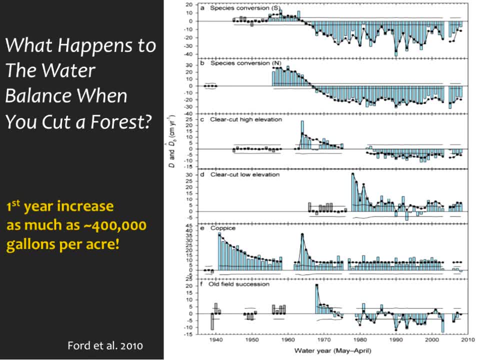 pattern: An increase in growth, but after the clear cut and the high elevation that stream flow is actually lower than the reference. whereas the low elevation clear cut is still higher than the reference, The top is forest: Increase, cut again and increase and then flow greater than the reference ever since. 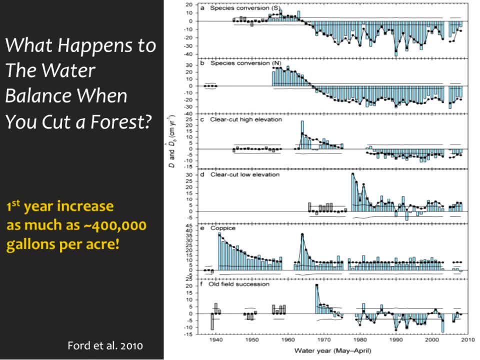 Old field succession, kind of all over the place. What this shows, the take home message here, is a couple of things. One is you can greatly manipulate the water balance by manipulating the vegetation. In all cases, what's happening is we're changing the structure and the species composition. 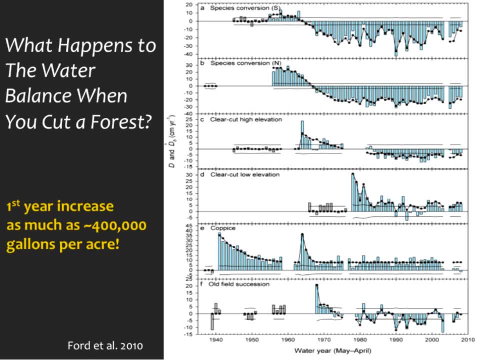 in the forest. In some cases that can be a fairly substantial change. In some cases that can be a fairly substantial change, As the example in the species conversion in the top two graphs. It's also interesting to note that in some cases we're now in the 40th or 50th year. 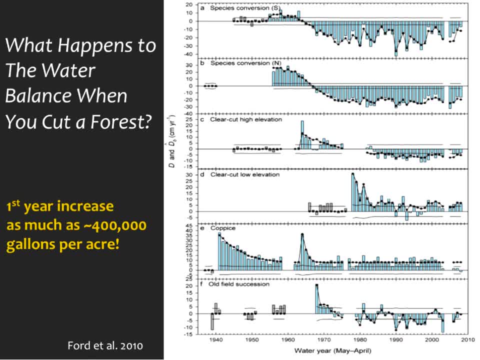 after cutting. in these experiments, and except for perhaps the old field succession, none of the watersheds have returned, from a water balance standpoint, back to what they were prior to the disturbance, prior to the cutting. So here's a second example. 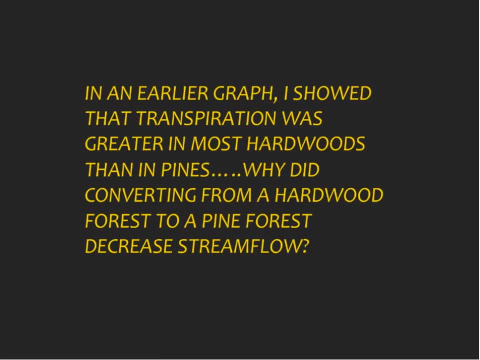 I'm going to show you a couple of examples. I'm going to show you a couple of examples. Here's a second question for you. Quick pop quiz number two. In an earlier graph I showed that transpiration was greater in most hardwoods and an individual. 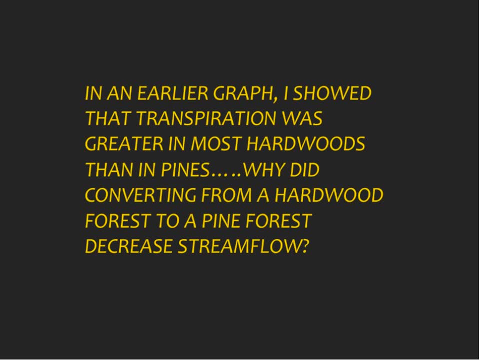 tree basis than it was in pines. Remember the pines and the yellow and the hemlock had among the lowest individual tree transpiration rates than any of the hardwood trees. Why did? in the graph that I just showed you, why did converting from a hardwood forest? 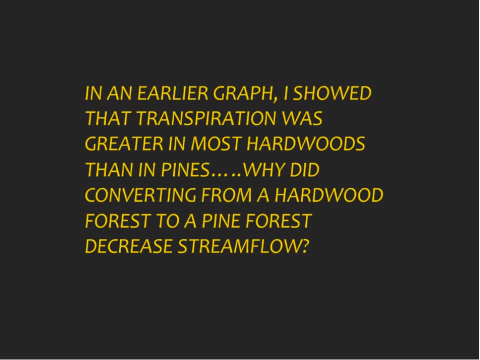 to a pine forest result in a decrease in stream flow. And if you have some ideas or guesses, go ahead and type them up in the chat room or just think about it and I'll show you the answer here on the next slide. 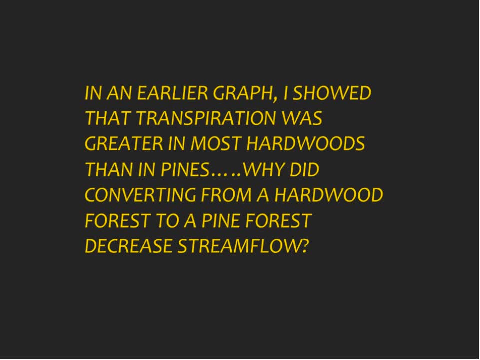 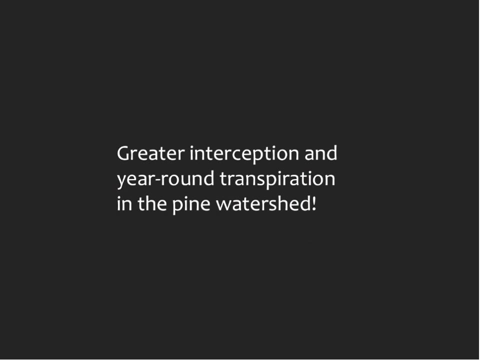 Okay, Okay, Okay, Okay, Okay. Any guesses All right? Well, the reason that's the case is that watersheds are made up of a compilation of individual species that create a stand, and that stand then had a greater interception. 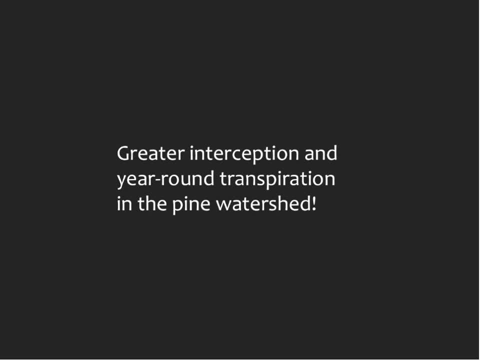 because of the evergreen nature of the pine forest and also had year-round transpiration in this moderate environment. Okay. So, even though at the individual tree level, in the middle of the growing season, the pines have a much lower transpiration rate at the annual level, in a well-stocked stand it. 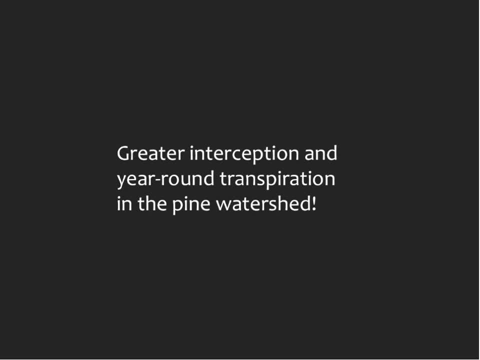 intercepted considerably more precipitation than was able to transpire year-round, with the moderate growing season typical of southern ecosystems. So what? this one of the take-home messages there is: what happens at the individual tree isn't necessarily what's going to happen when you scale up to longer time. 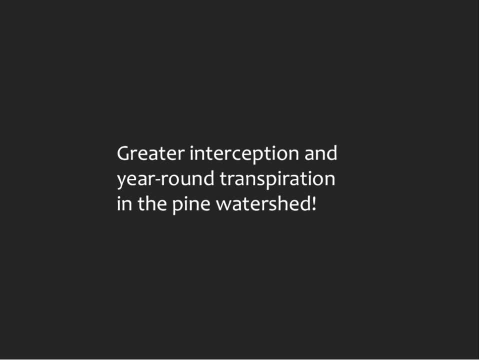 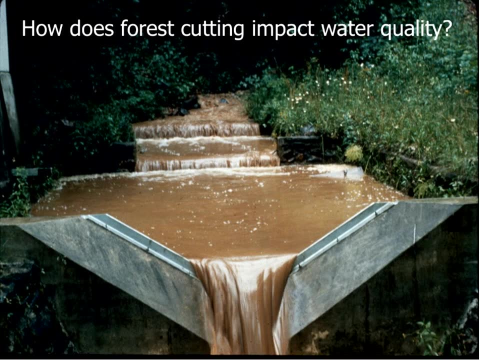 Okay, When you scale up to longer time frames and larger spatial scales. How does forest cutting impact water quality? The other thing again that we talked about- the value of a forested watershed- is providing very high quality water. Well, what happens when you manage the forest in terms of water quality? 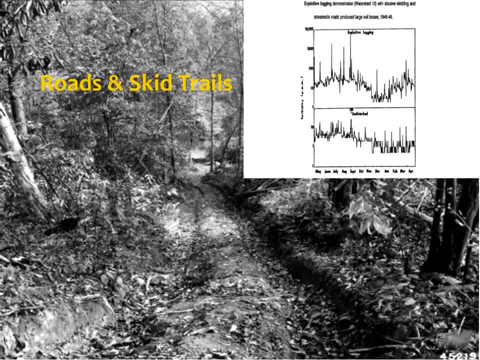 Well, unfortunately, there's a long legacy of bad examples of how managed- or, in this case, cut forest. I wouldn't even call it managed forest, It's just that it has negative impacts on water quality. The upper right graph is- you don't need to see the scale on it, but essentially in some 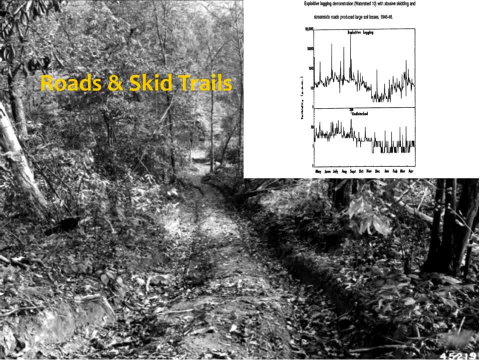 cases a 10,000-fold increase in sediment or turbidity. as a result of very poor logging practices And in the old days before we were enlightened and roads were built correctly, a lot of the skid trails and roads would go right up and down a watershed or be placed right alongside. 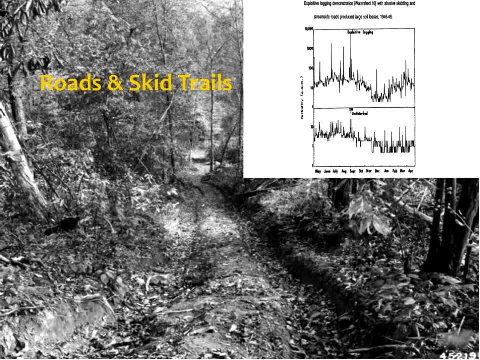 the stream. Okay, So there's a clear concern for the impacts on water quality And, as I noted earlier, on the most vulnerable and most important component of the watershed and the area where we'd expect most overland flow erosion and sedimentation comes from. 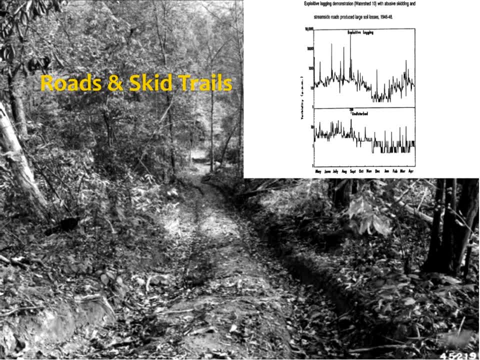 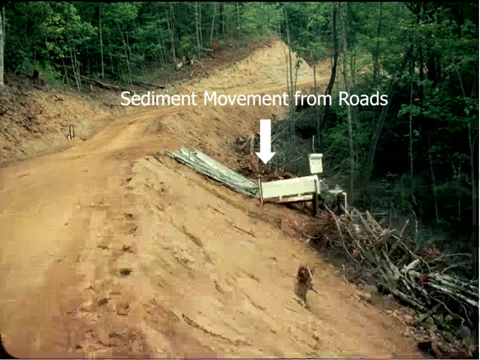 these roads and skid trails. So there is a legacy and a history of high sediment and poor water quality as a result of what were, at the time, very poor land management practices. Now we've come a long way in our knowledge about how to properly build forest roads. 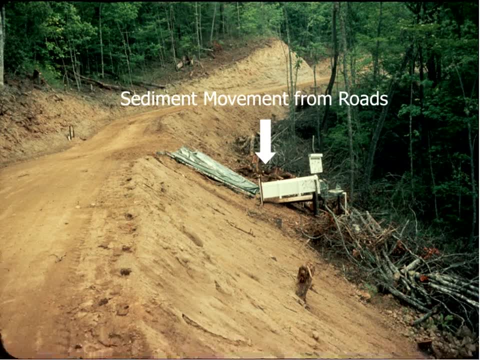 and how to minimize the sediment movement from those roads when it occurs. And a lot of that has come from research and also on-the-ground experience. Instead of building roads up and down the watershed or right next to the stream, build them along the slope, pay close attention at road crossings, et cetera. the kinds of 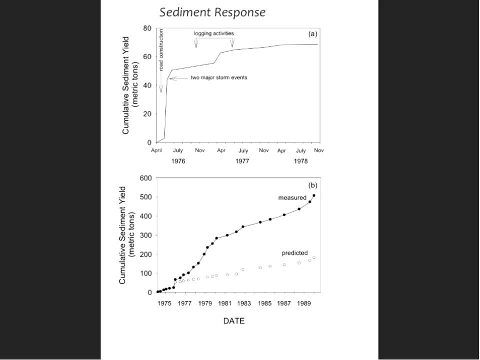 things I talked about before, And the bottom line is is that when best management practices are in place and in terms of sediment from forest, road building or forest logging, those activities are compatible with protecting water quality and reducing sediment and turbidity in streams. 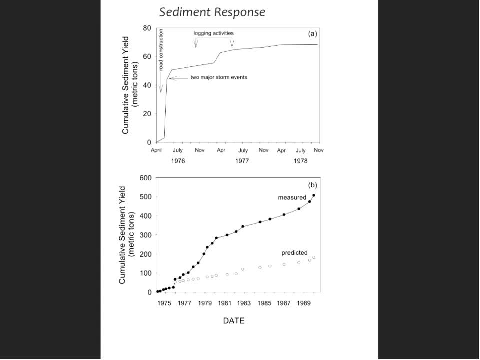 It's not necessarily zero. this is an example from some of the studies at Coweta that showed that there are some vulnerable time periods where if you get a bad consequence here- in this case, two major storms occurring right after road construction- you can still get. 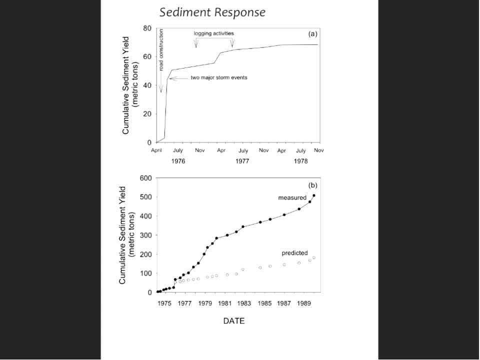 some sediment pulses, But for the most part those activities were very short-lived and the rate of sediment production was essentially comparable to the reference. So forests can be managed in ways that predict or protect water quality from a sediment. Thank you From a sediment standpoint. 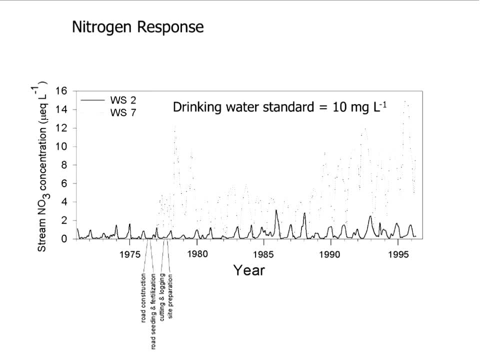 From a nutrient standpoint, there really is not much of an issue. This is a graph of a log watershed at Coweta. The units here are microequivalents per liter. The drinking water standard is about 10 milligrams per liter. These are orders of magnitude lower than the drinking water standards. 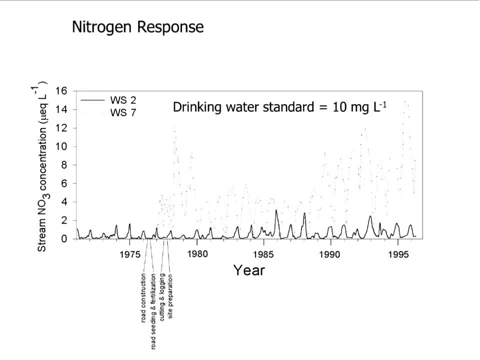 The lower solid line that you see there is what comes out of the reference watershed. Those are levels that are right at the detection limits because forest ecosystems essentially take up all the nitrogen that they can, especially in southern ecosystems. The fainter blue lines that you see are what happened on the log watershed, and it's higher. 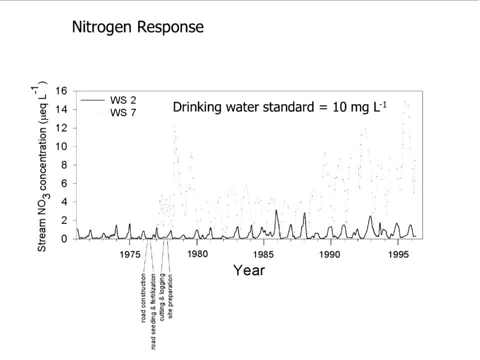 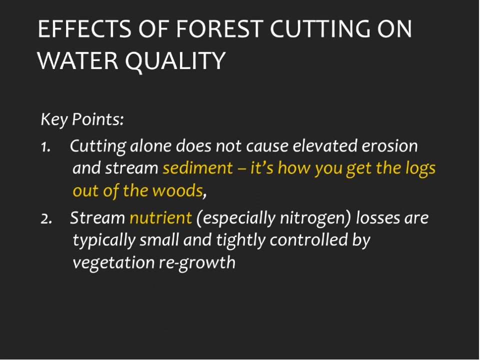 and you'd expect it to be higher, because you are disturbing the system and stimulating nutrient cycling processes, But and also there are some changes in species composition that may occur. I'm sorry, I'm sorry, I'm sorry, But But the levels are still very, very low and well below drinking water standards. 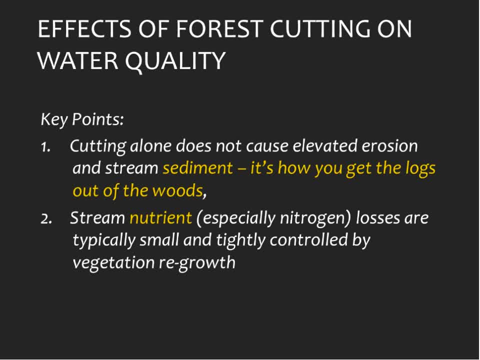 So the summary of this is in terms of affects, not forced cutting on water quality. some of the key points that we know is that cutting alone does not cause erosion and stream sediment. It's how you get up the logs out of the woods. so very careful protection of roads. 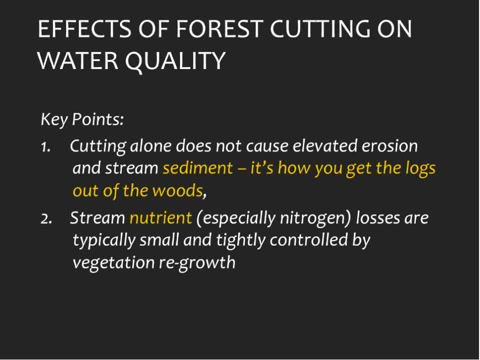 If you work while torrentially, there's a lot of lost cores that have drifted off, So you just pressure So very de Shane And stream crossings, skid trails et cetera, you can log without elevated sediment. 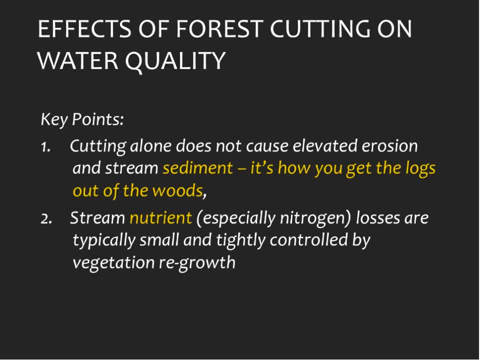 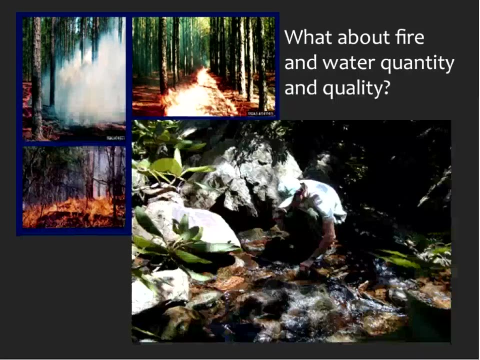 And stream nutrient losses are very, very low and tightly controlled by that vegetation regrowth which takes up any of that nitrogen or nutrients that are mobilized. What about fire and water quality- One of the- and quantity. I'm going to talk primarily about quality, but also quantity. 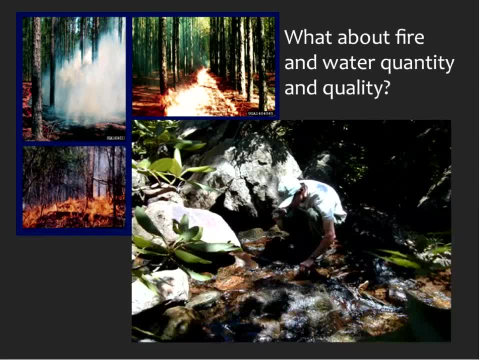 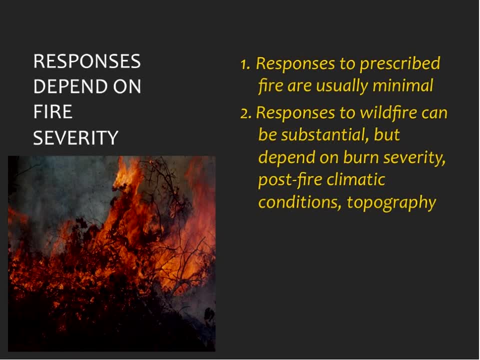 Prescribed fire is a common management tool in the south and increasingly used in other places for protection from wildfire or wildfire risk. One of the things that we've looked at in quite detail across the south is what happens in terms of water quality and quantity when you fire, when you use fire. 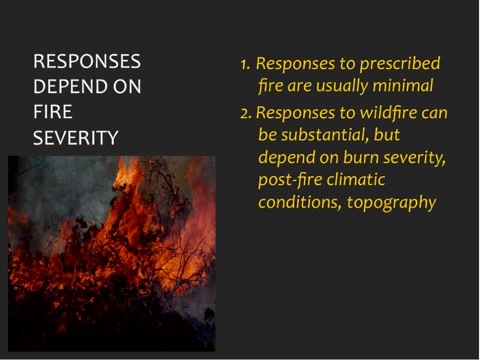 And what we find is that the response depends on fire severity, And responses to prescribed fire are usually low, Usually quite minimal, because severity is low, Responses to wildfire can be substantial, especially ones that are have a high fire severity or burn severity coupled with big storms that might occur immediately after. 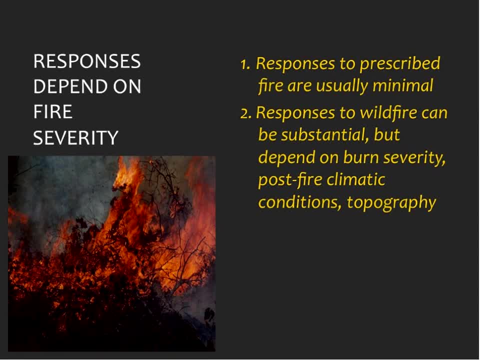 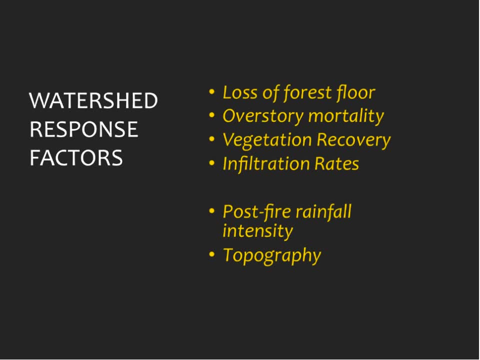 a severe fire and in areas that have steep slopes and rough, complex topography And the types of factors then that influence watershed, response is going to be how much of the forest floor you like, How much you lose as a result of a severe fire. 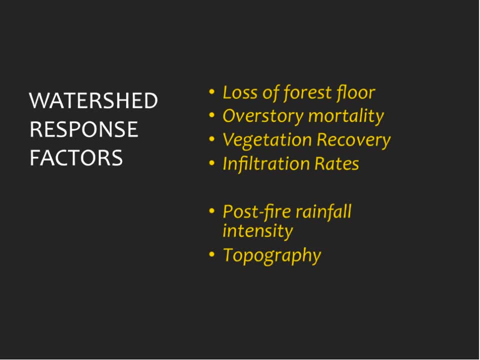 How much overstory mortality occurs, How fast the vegetation recovers, How that impacts infiltration rates- In some places in the United States you can actually get some hydrophobic soils created as a result of fire, which lowers infiltration rates- And then some things that you can't control, like post fire rainfall intensity and topography. 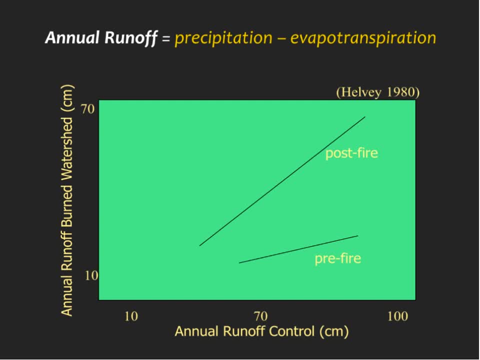 This graph here essentially shows, for some southern forest ecosystems, Especially ones that had a very high mortality level, What happens to annual rainfall or annual runoff, sorry. And the lower line shows the relationships between a control watershed and a burned watershed before the fire. 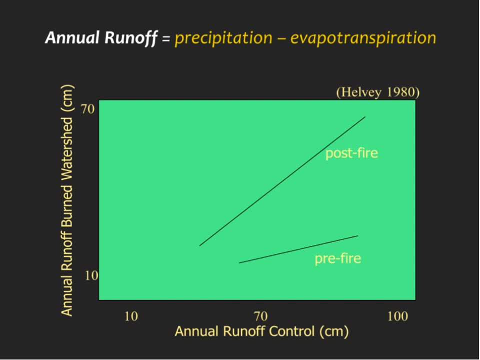 So for 70 inches of runoff from one watershed, you've got about 15 from the one that got burned fire. there was a significant increase in the amount of runoff from the burned watershed and that was directly related to the fact that this was a watershed. 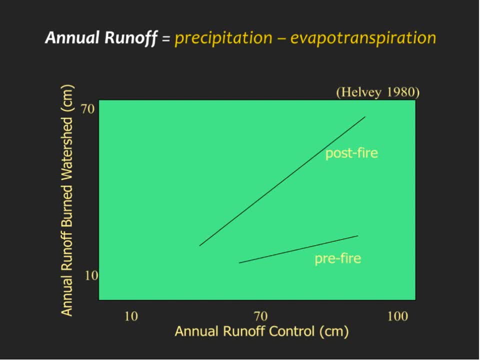 that had high mortality. about 50% of the trees were killed and, as a result of evapotranspiration was reduced and annual runoff increased. Now this is this can happen and is typical in wildfire situations. very rarely would this occur, if ever, in a prescribed fire situation. Same is kind of true with 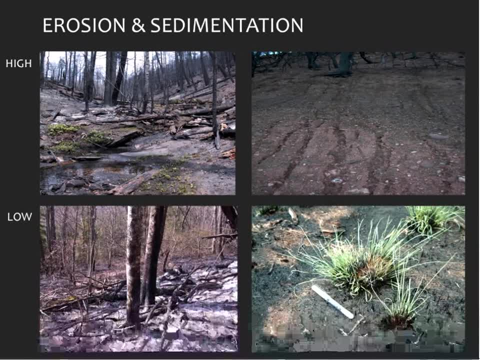 erosion and sedimentation. where you have high severity typical of wildfires, you get what occurs in the upper graph: high tree mortality, the complete loss of forest floor and, with post fire storms, considerable amount of ash wash and surface erosion and rill formation. The lower part of the graph is more typical. 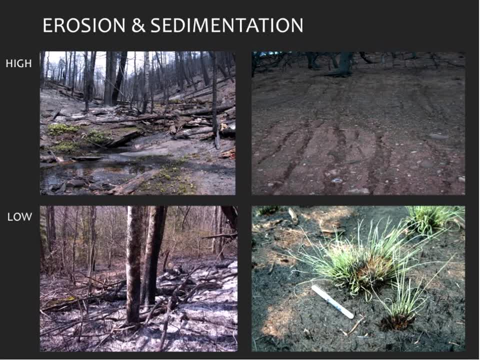 of a prescribed fire situation. The lower part of the graph is more typical of a prescribed fire situation. The lower part of the graph is more typical of a prescribed fire situation where you still have live trees, you still have quite a bit of coarse woody debris and, as the lower right hand panel shows, you might even still have. 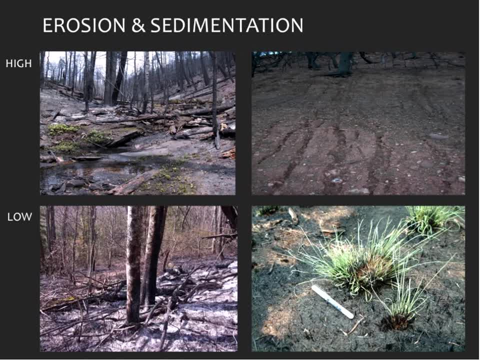 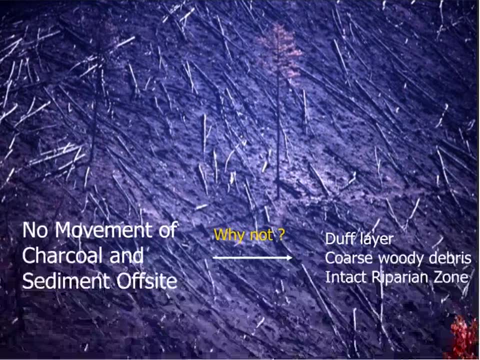 understory vegetation and forest floor left. Now you don't need a close-up view. here's an example of a very large watershed that was severely altered as a result of forest cutting. in this case, a high intensity- not high severity, but a high intensity fire that consumed a lot of the. 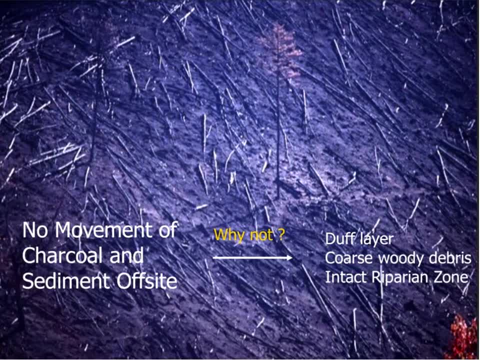 ground material. but this experiment showed absolutely no movement of charcoal or sediment off-site. and why did that not occur? well, really, for three factors. one is: this was a high intensity fire, but not a high severity fire, so the dust layer was maintained. as you can see in the picture, there's a lot of coarse. 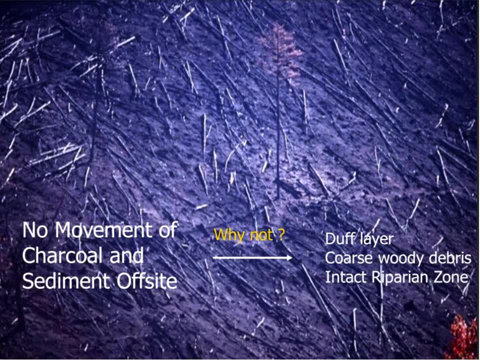 woody debris that could act to trap any charcoal or sediment that flew, that that flowed off of the site in high, intense rainfall events. and this was also a watershed that had an intact riparian zone that didn't burn and anything that would have would have flowed in small areas through this burned area would. 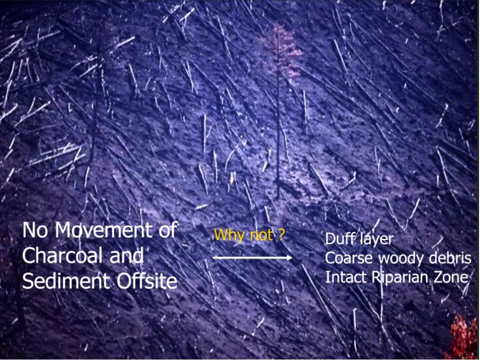 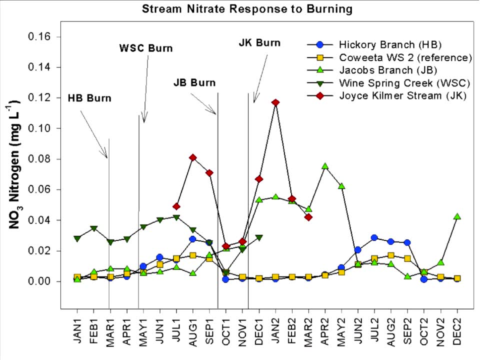 have been trapped and stored in that riparian zone. Same is true in terms of stream nitrate response to burning. only in the most severe fires might you get a nitrate response, but for the most part levels are incredibly low. again, drinking water standards is 10 milligrams per liter. 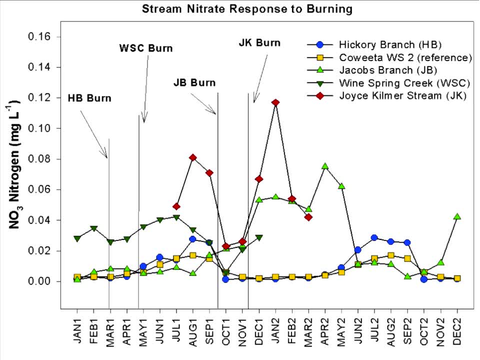 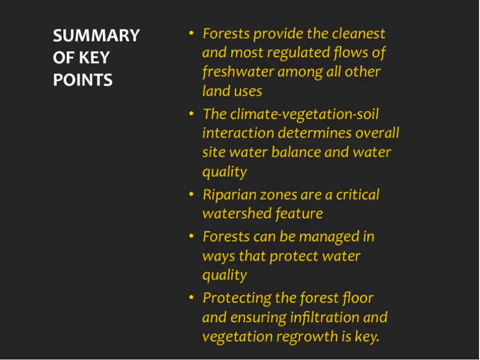 This is a bunch of different fires that have occurred, in this case in western North Carolina. some of these are even wildfires and in no case, while you might see a small increase in stream, nitrogen levels are always very low and well below drinking water standards. Okay, so I'm just going to summarize here and hit some key points, and then I'll see. 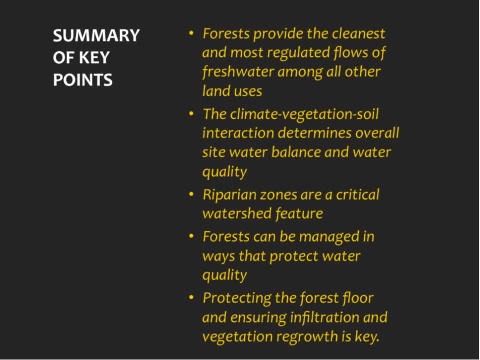 if there's any questions after that. So my key points are as follows: Forests provide the cleanest and most regulated flows of fresh water among all land uses, due to decades of research. this is a statement that is quite I'm quite confident in and, as the National Research Council said, it's settled. 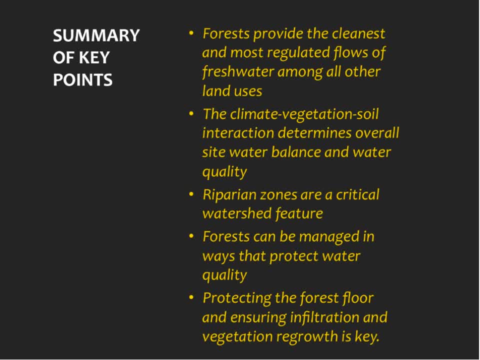 science. That relationship is determined by the climate, vegetation, soil interaction, which determines the overall site water balance and water quality. that can be manipulated to either increase or decrease flow as a result of disturbance or management choices which either change age, class or structure or change species. it is, it is, there is enough in that. 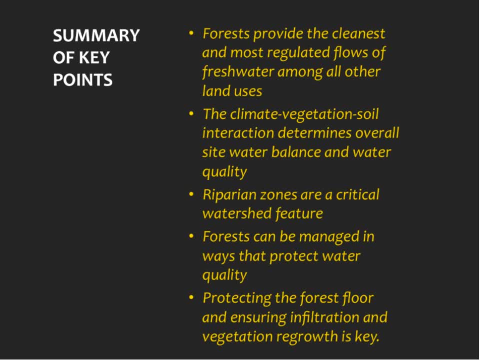 relationship. that flow can be either increased or decreased depending upon management activities. Riparian zones are the critical watershed feature. they're the place where sediment and nutrients are trapped as it flows from the upland to the stream surface water zone. And having a healthy, functioning riparian zone whose width can be determined by a variety 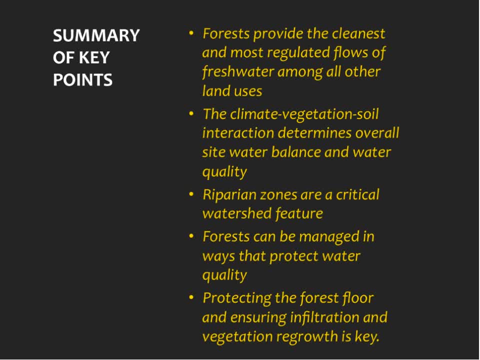 of factors is a critical part for maintaining water quality. Forests can be managed in ways to protect water quality. paying attention to keeping the forest floor intact and ensuring infiltration, and having a rapid vegetation regrowth is some of the Practices that can be implemented in order to do that. 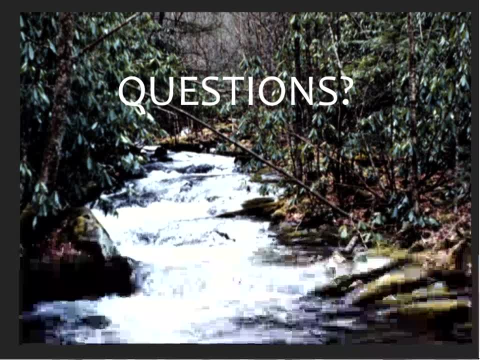 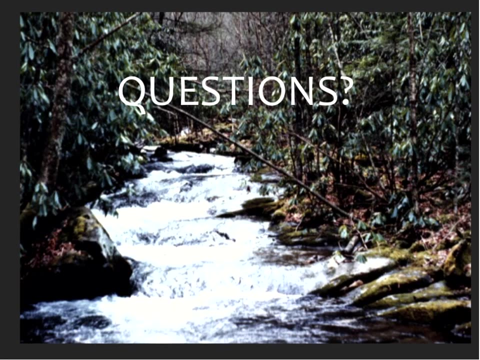 Okay, so that's the material that I wanted to cover in my hour. Be happy to answer any questions through whatever process is used here to do that. Bill Great thank you, Jim. that was a fantastic overview and just a reminder, folks. this will be archived too, so that if there's any information that 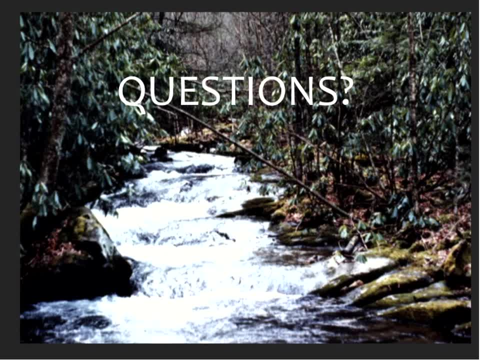 You feel you need to go back over. we'll have it up online in the next next few weeks or so. do we have a question? Rebecca has her hand up. Rebecca, let's see. I'll give you audio permission or, if you'd like, you can go ahead and chat your question in. 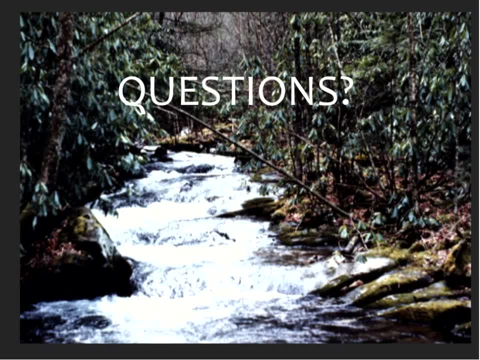 You should have audio permission right now. Okay, I guess I'm not sure if she has a question or not, Jim. Okay, In the meantime, while we are going through this, I'm going to push out a U R L That will allow you to take your quiz and obtain your credit. hopefully it's redirecting as we speak here.